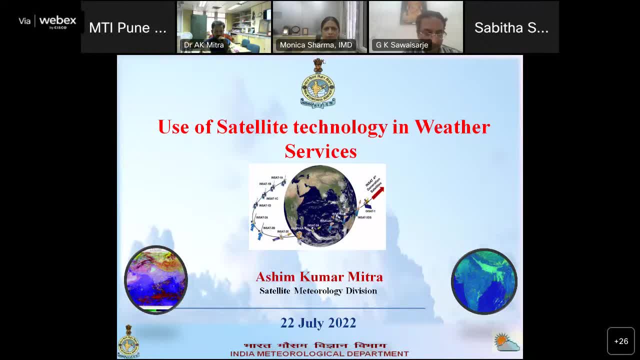 and obtained his PhD in quantitative application of remote sensing in weather forecasting- remote sensing in weather forecasting- from Jadavpur University, West Bengal, in 2014.. He has 19 years of experience in satellite metrology. He was instrumental in utilization of INSAT-3D-3DR satellite data in RGB preparation, disseminations and NWP assimilation. He was 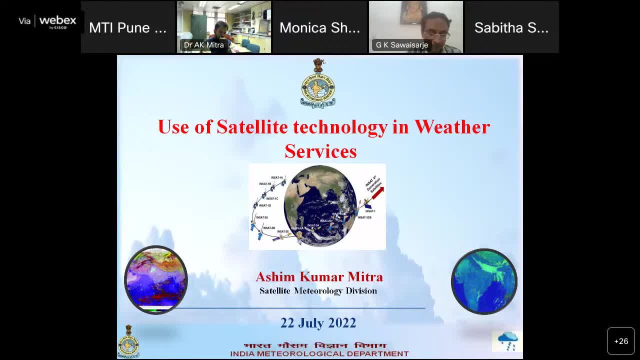 awarded the MoEAS Award 2015 of Certificate of Merit for his outstanding contribution in the field of atmospheric science and climate change. He is also heading geospatial group of IMD and has made available various products to forecasters and stakeholders. He is also 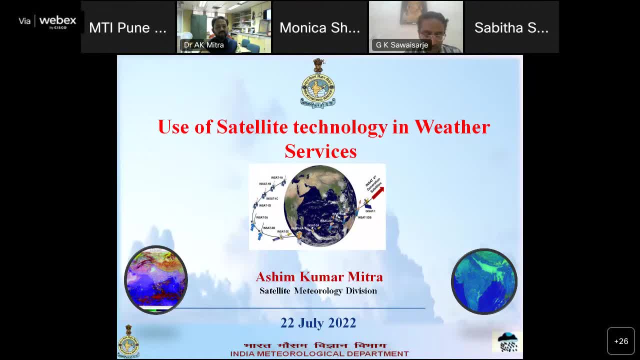 engaged in research work in operational metrology, atmospheric science, since last decade, Dr AK. So I now request Dr AK. I now request Dr AK Mitra to continue his lecture and to the participants for their queries in chat box after the lecture. Okay, 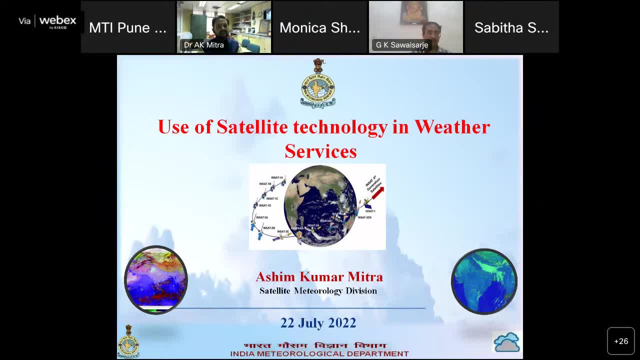 Dr AK. Thank you, Savai Sarjiji, for introduction and providing me the opportunity today. So good evening all of you. Today I will give you a talk in the use of satellite technology in weather services. So I think my slide is: 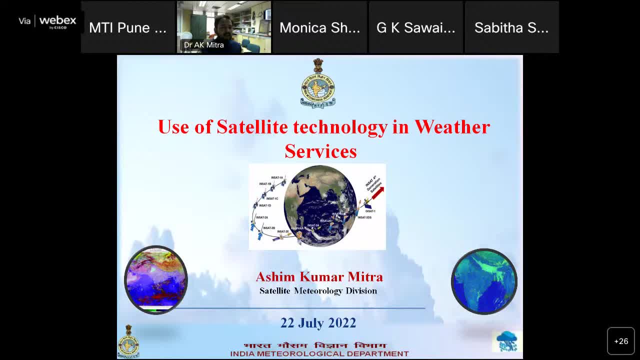 visible to everybody. Dr AK, Yes, Dr AK, Yes, sir, Dr AK. Okay, And my voice is also audible to everybody. So let's start with today's lecture. So first I'll just give you the brief which is very common to everybody, that where 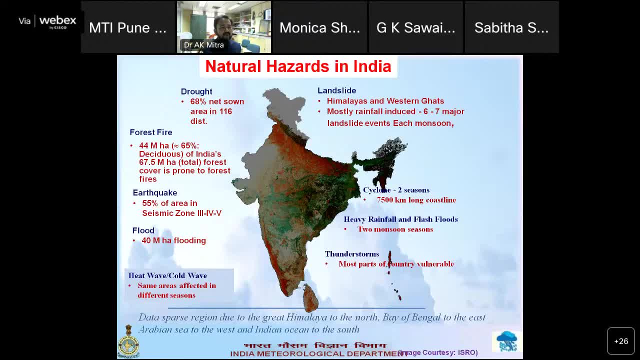 the natural hazards in India basically finds. So if you go by, there are a number of areas like they need to cover, like 68% net shown area in the drought region, forest fire, there are 65% of Dr AK. Similarly, earthquakes, flooding, thunderstorm, heavy rain. 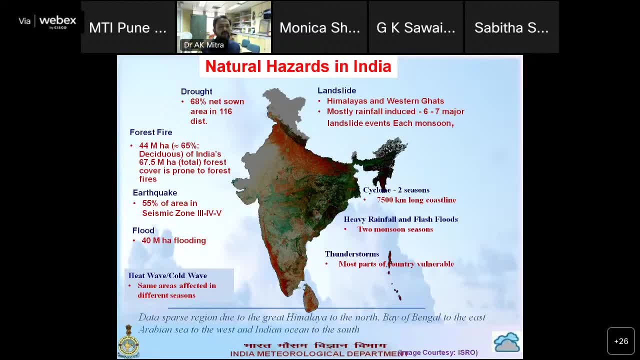 flash flood, landslide, heat waves, cold waves. So we have all been gathered with the kind of a natural hazards in India since so long. Basically, if you can see the data sparse region, particularly due to the great Himalayas, to the north Bay of Bengal, to the east and Arabian Sea. 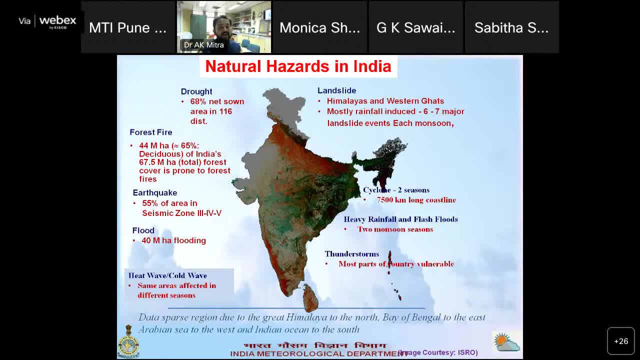 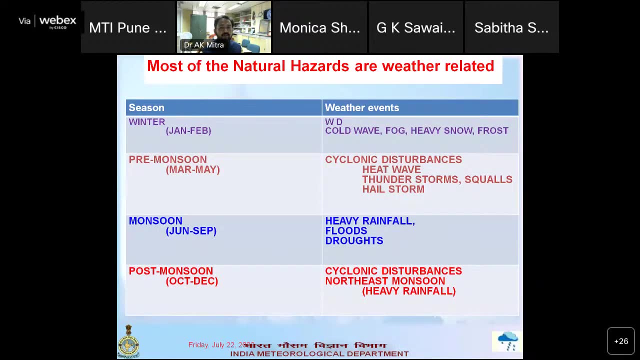 to the west and Indian Ocean to the south, So large area which we are finding out that there are site of kind of information is required And there we feel that some observational point of view we need to gather those information because we have a number of natural hazards in a different 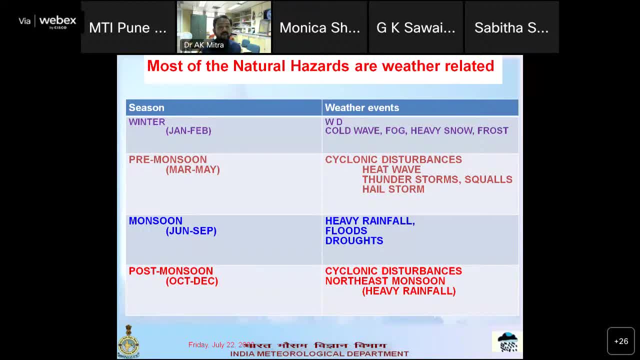 sort of weather related events And they are seasonally dependent, Like, if I can say, the winter month, mainly cold, wave, fog, heat and western disturbance, heavy rain, And then, if I go to the pre-monsoon season particularly start from March to May, cyclonic disturbances, heat. 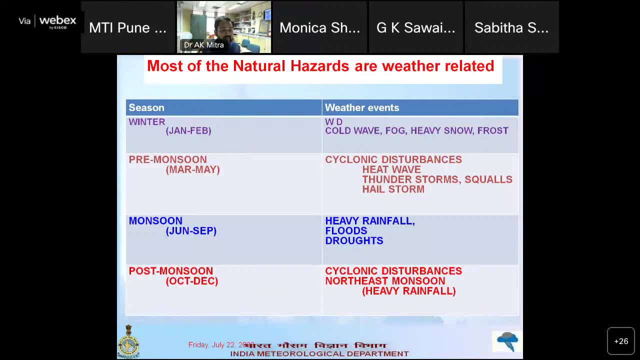 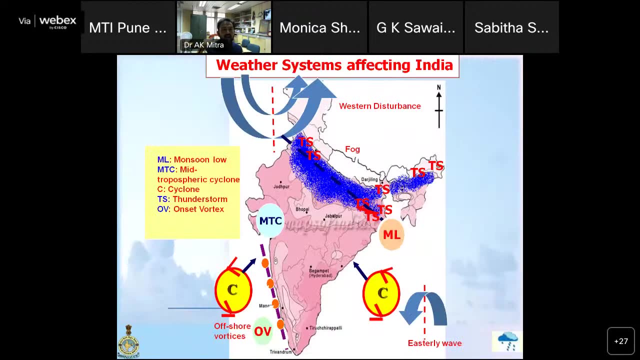 waves, thunderstorms, falls, hailstorms and then monsoon that we are currently facing that- heavy rainfall, floods and some time, And then post-monsoon, that is, October to December, cyclonic disturbances, northeast monsoon, heavy rainfall. So, basically, how our weather? if these 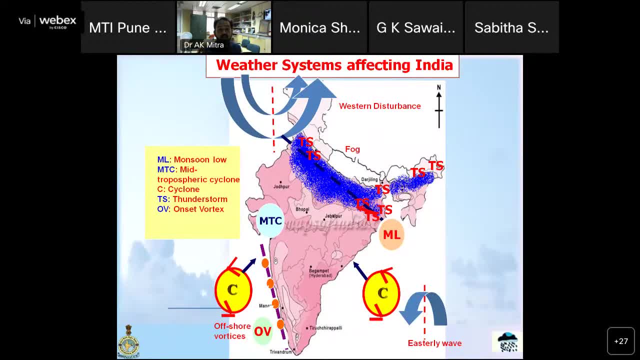 systems are affecting India because it is not homogeneous to everywhere. Sometime you can, you will be finding out WDs, mainly over the northern side. At the same time, MTC, mid tropospheric cyclone- those circulations are monsoon low Or you can say mid tropospheric cyclone, that you can. 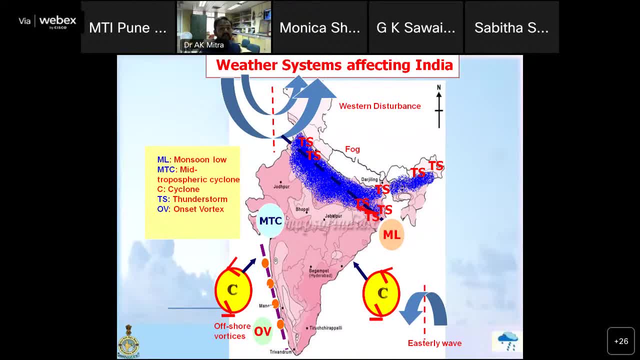 see they have Gujarat coast and that we have a experience recently. And then thunderstorm entire India, and then onset vortex that will be near southern- you can say southern- parts of country. This is you can see- And then Arabian Sea and Bay of Bengal circulations, that is, cyclonic circulation for cyclonic agencies. And then 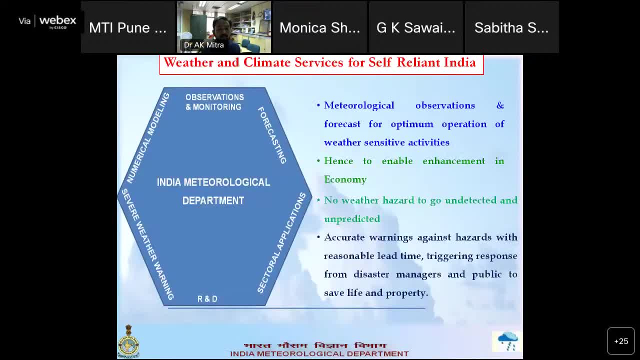 these are the kind of a weather system we are affecting our country, But metallurgical observations are mainly enabling the best part of it, that we can able to detect it, because it enhance in the economy sector also. So our target will be like: no weather hazard should go undetected. 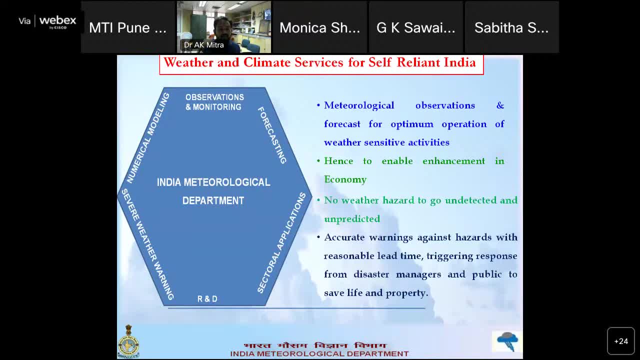 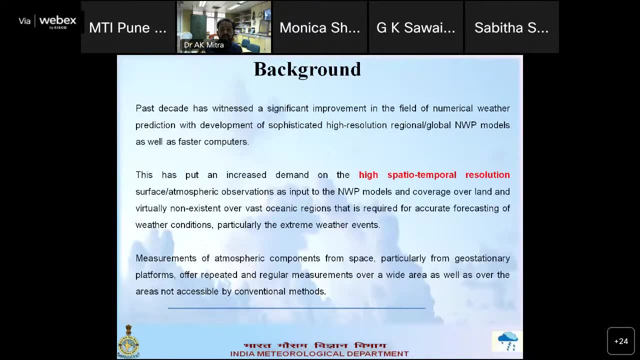 and unpredicted. So the main aim of our organization is, which has to be accurate warnings that can hazards with reasonable lead time, triggering response from disasters managers and public to the same life, to the property, And that is the most important part. Then, if I can go, 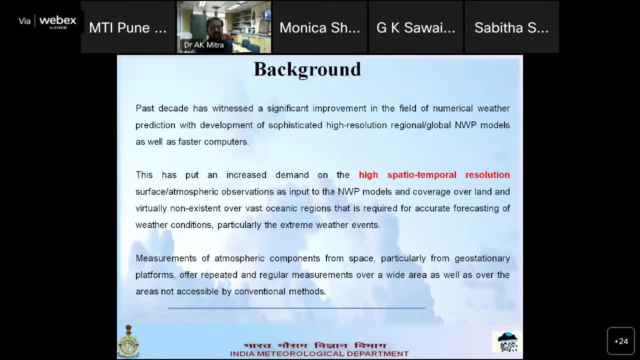 with the past decade we are to witness, with a significant improvement in the field of prediction And development, sophisticated high resolution model and WP models, as well as faster computers. But still this has put an increased demand on highest spatial temporal resolution, surface atmosphere observation as input to the NWP models and coverage over land and virtually 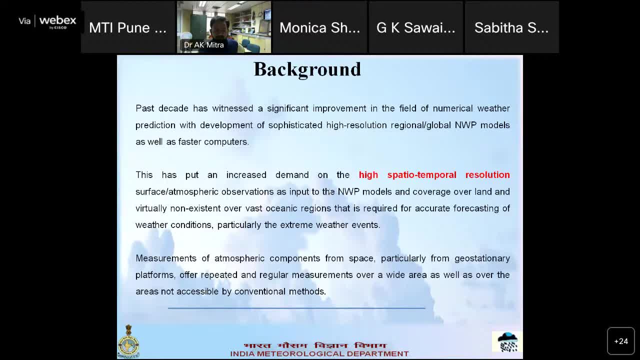 non-existent over the vast oceanic region, As I mentioned, over Arabian Sea or Bay of Bengal and Himalaya. So they required accurate forecasting of weather condition with all those information, particularly dealing with the kind of extreme weather events, So the measurements of atmospheric component from space here plays. 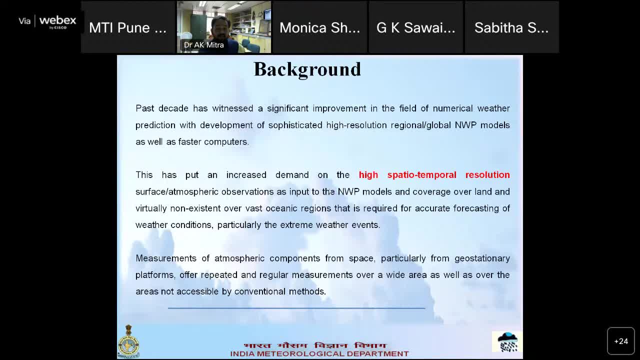 a very important role, That is, a remote sensing, that I will say, particularly from the geostationary platform, where repeated information, repeated observation, with a regular measurement over a wide area as well as over the area that is not accessible by conventional method, as I mentioned. 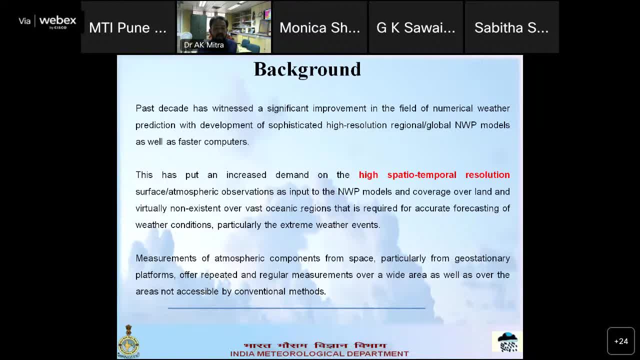 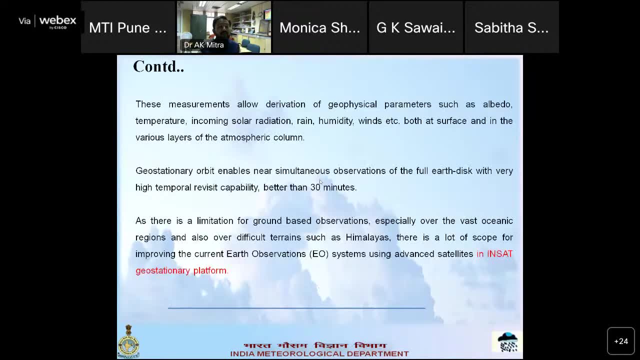 that like Himalaya and the ocean. So here a reliable observation will be from the component is called the space based component. The space based component basically is a number of parameters will come out from the space based, that is, from satellite, or you can say the remote sensing, So like temperature incoming solar. 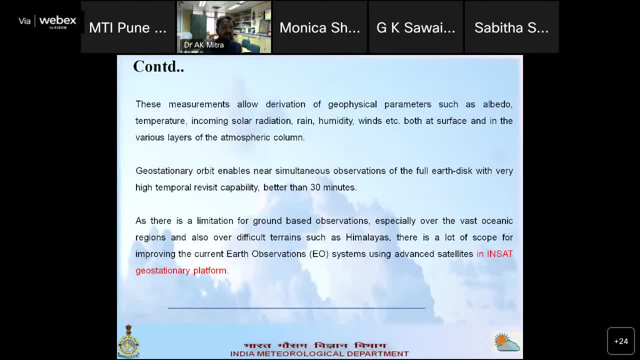 radiation, rain, humidity, winds, both at surface and in the various layer of the atmospheric column. So, as I mentioned, that geostationary orbit, what basically it is? it is a basically enables near simultaneous observations. So observation with the full earth disk with every every half an. 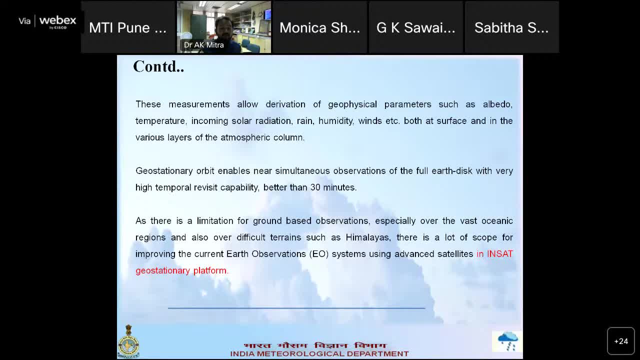 hour, every 15 minutes. So with the higher temporal resolution uh, with the very uh, we can say, the capability of scanning the uh as and when we require that information comes from the geostationary orbit and, as there is a limitation of ground-based observation, as I mentioned, that those area where we cannot take observation because of the um 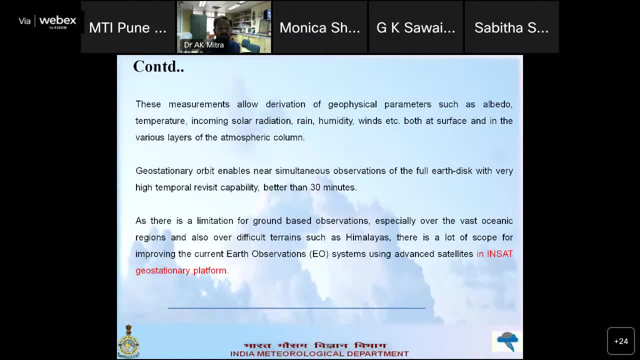 data spar region and then over the vast oceanic region and mountainous region and difficult terrain like Himalayas. So there is a lot of scope for improving the current earth observing system that is called remote sensing capability system with advanced satellites, particularly that what we are, we are, we are from almost like 50 years now, from 1982 or what 40 years? 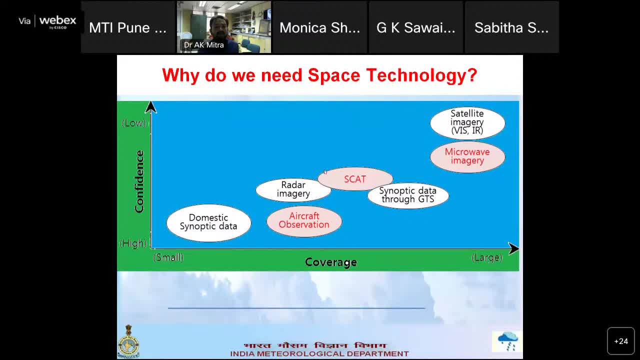 that is inside geostationary platform. So so here comes that: why do we need space technology? as you can see the graph, uh, if we go the domestic synoptic data, it is very small and and but it is the location specific, so you cannot have a um that is there is, confidence is very low, but 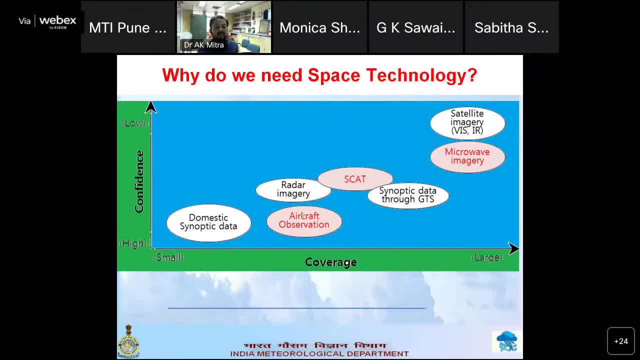 small locations, as your coverage areas are, goes slowly, slowly. our confidence limits are getting so as you go to the imagery visible, IR. so now we need to bridge that gap with the number of observation from the space point of view. so so basically, what is the remote sensing? now I will. 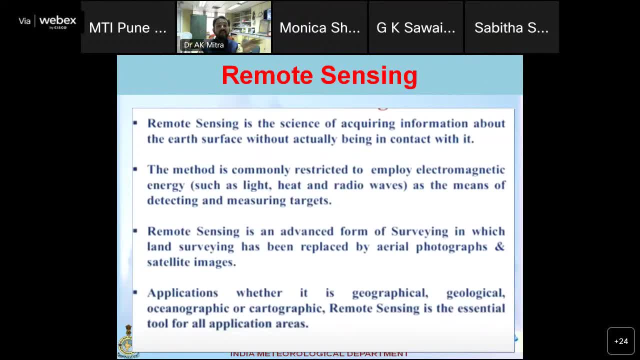 come to the, to the talk of how remote sensing plays and bridging the gap of the higher confidence of the forecasters so that we can- we can deal with the number of weather hazards. so remote sensing is the same: the science according information about the earth surface without actually being 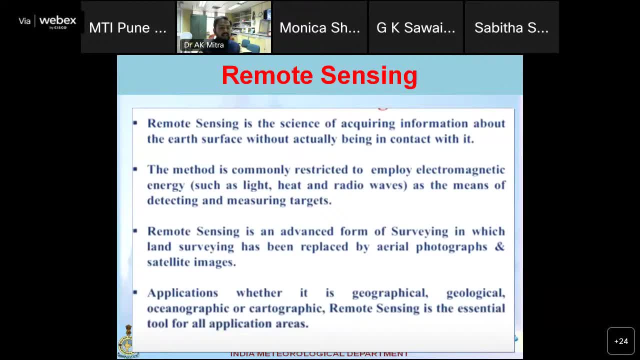 in contact with it. so we can take this observation from long, and then the method is basically to restrict it, to employ electromagnetic energy such as light heat, radio waves, and they because the means of detecting the measuring targets. so remote sensing is an advanced form, surveying in which land 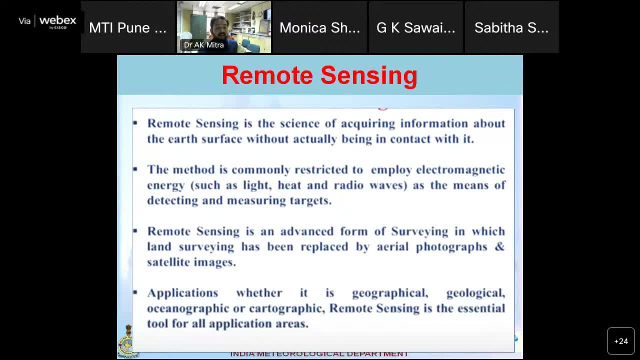 surveying has been replaced by aerial photographic and satellite images. so we are not going by the place to plan, it is taking from the high observation, or you can take it from the space, and it is replaced by the satellite images. so so the what will be the application and that then 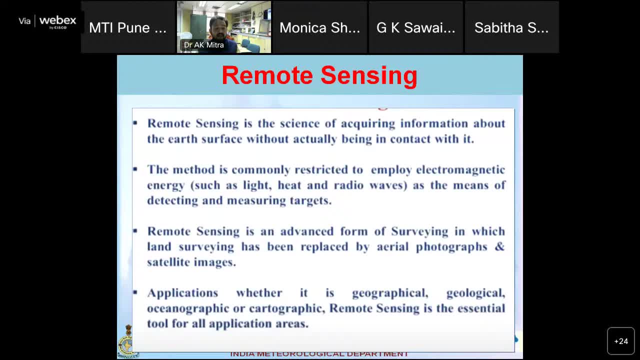 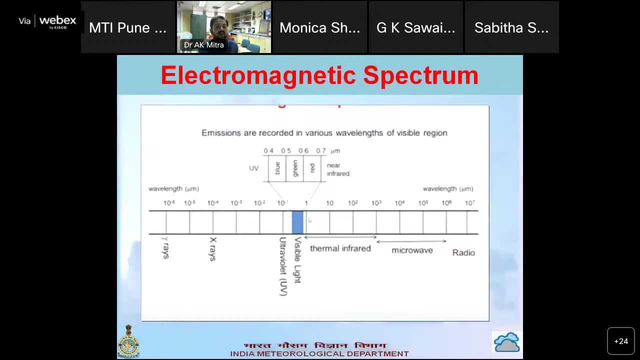 application is geographical, geological, oceanography, graphical cartographic. so these are the kind of application that we need to uh with to deal with so remote sensing here, essential tool for application area like, like, as I mentioned again, geological, oceanographical, atmospheric cartographic. so these all information come under. 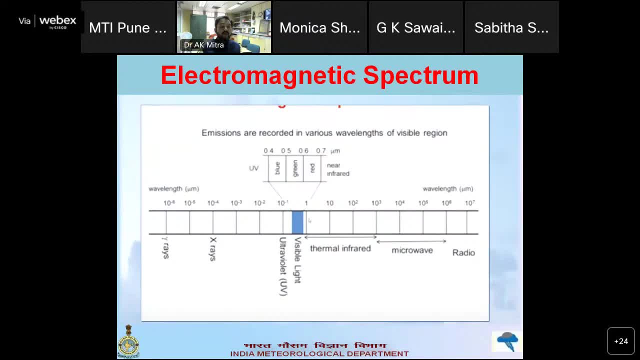 the electromagnetic and electromagnetic spectrum. so, as you can see that what, whatever emissions are recorded in different wavelength and visible region, you can get it like you can see. first you will see there is a radio frequency that we do not need for the atmospheric science and weather. then it comes to the microwave. microwave, you can see 10 to the power to 10 to the power, 6.. 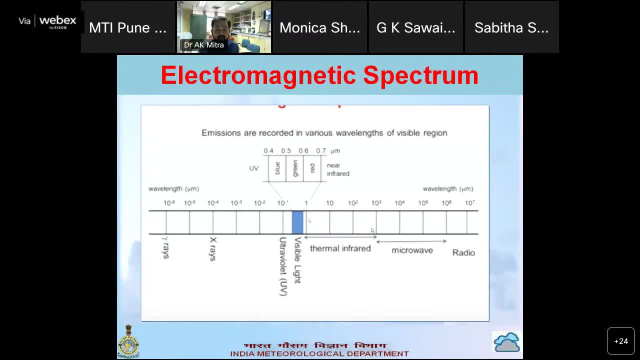 so here it is. it is a long, very longer wavelength. and then comes with a thermal iron, like you can see, 10 to the power minus 3, and then visible light. you can see here. in the visible light you can get the near infrared. you can see blue, green, red. so these are the micrometer. that is the wavelength. 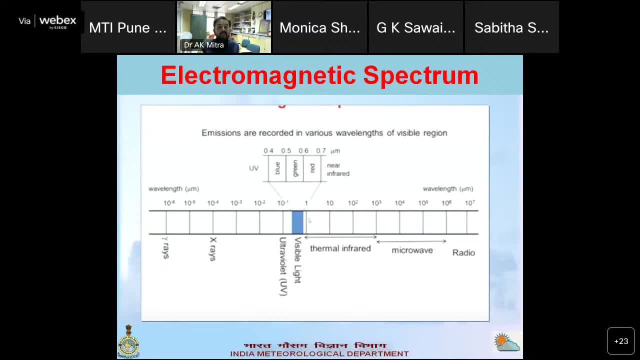 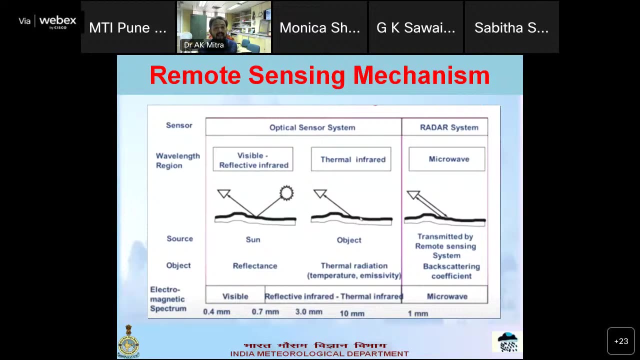 that basically says they send the emissions and basically they, they govern, or they are the medium where, the where, from the surface, and they are reaching to the satellite sensors. now, when they are reaching to the satellite sensor, how, um, what could be the mechanism like then? there will be two options like: what could? 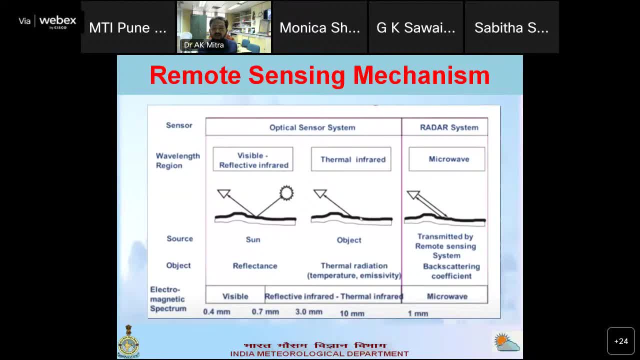 be the sensor wavelength, sources, object and what particularly electromagnetic spectrum where these observation matches like optical sensor system and we say so, we will be having a two-way visible reflective infrared and thermal iron. thermal iron- you can see here, uh, first object, where thermal radiation, temperature emissivity they are coming out from the your, your earth or skin of the earth. 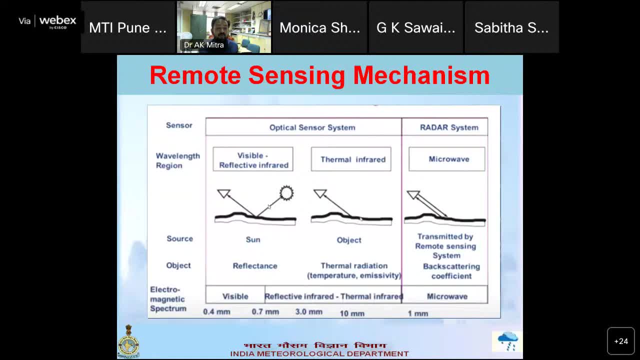 whereas visible reflectivity, basically whatever uh source of energy comes from sun, it is reflected back. so this reflection is basically taken care by the visible. so that object, this is the object and here it is a matter of. so you can say the object will be from visible wavelength, will be sun. 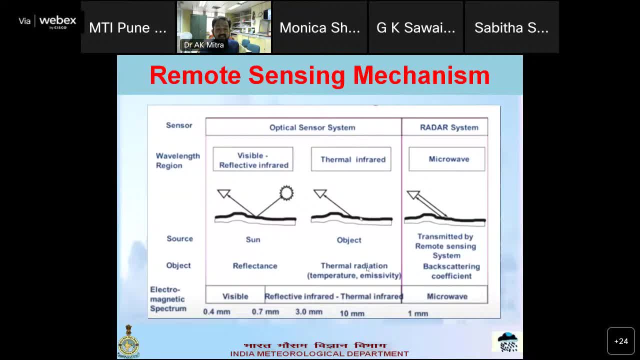 and the, and the object will be reflectance. so for ir, it is a thermal radiation, and then for visible is now, uh, then electromagnetic spectrum. what could be the better one? then visible channel, that is 0.5 to 0.75- you can see here- and then ir, 3 millimeter to 10 meter, 10 millimeter. so these 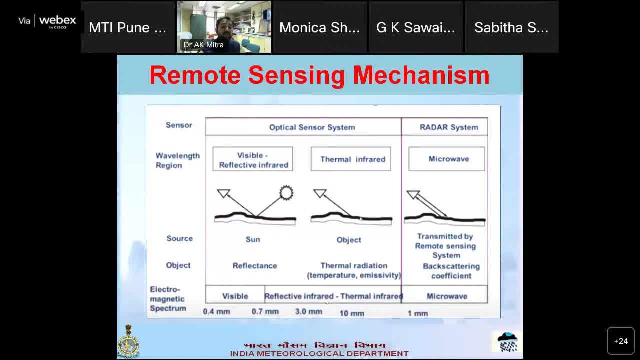 are the electromagnetic spectrum where you can. you can see the observation of tir and visible, so 0.4. and then it comes to the microwave. now, when we come to the microwave column, you will be finding how radar system is there. so microwave also. it is going up and going down, so it is a both. 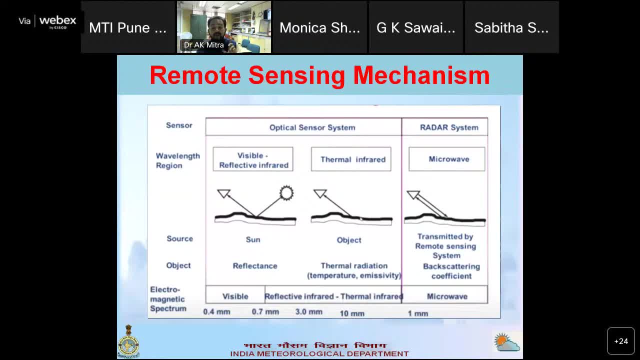 so it is active, sensor and passive, both the way you can get the microwave observation because it is transmitted by remote sensing system, one way of backscattering coefficients. and that comes with the one millimeter. so now you can see they have the entire range of electromagnetic spectrum. how 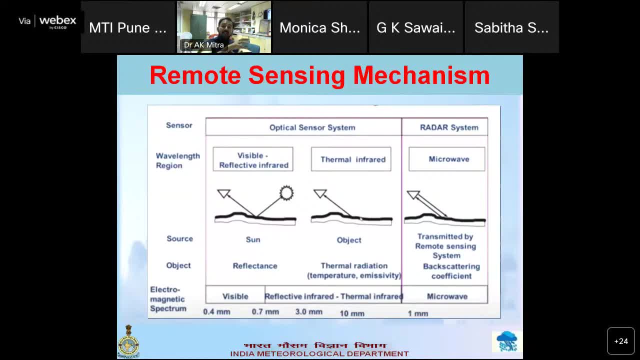 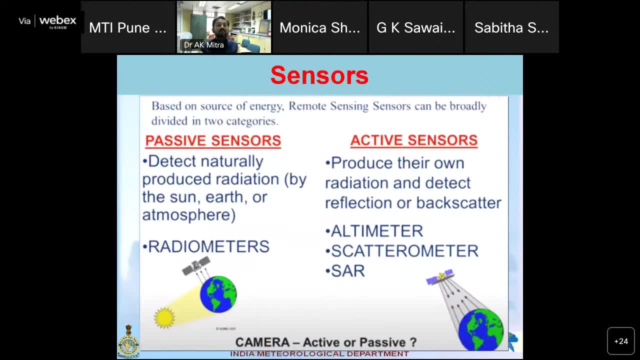 your uh satellite sees the observation over the earth. so, if we can, if we can go by the, the most important part is source of energy, how these based on source of energy you can get it then that that is what you need for the information coming out from the terrestrial radiation, or you can say, from the earth. 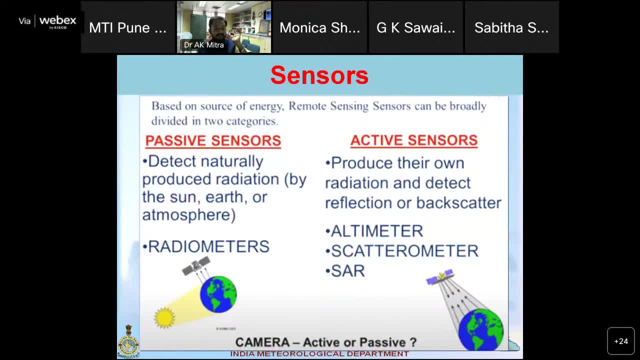 and the different layers of the atmosphere, see the cloud or other constituent gases, and the source will be either earth or sun. but where the active sensor- basically you know, like radar, sending the pulses beam and that is reflecting that that would be calculated, means you are sending the beam to the particular object so they produces their 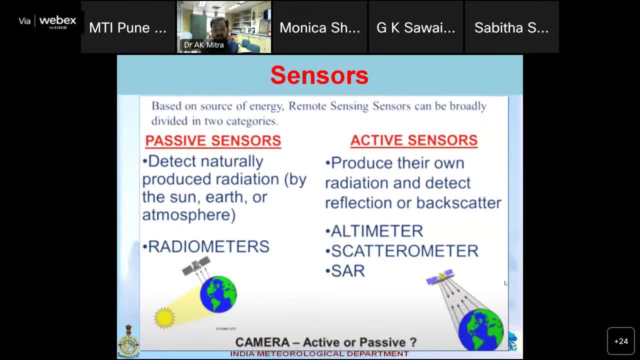 own radiation and detect reflection or back scatters, as you can see in the image. so some examples like altimeter, scatterometer, sar, so saris, uh aperture radar, synthetic aperture radar- this is sar is most important- and they are basically meant for a kind of observation which is very high. 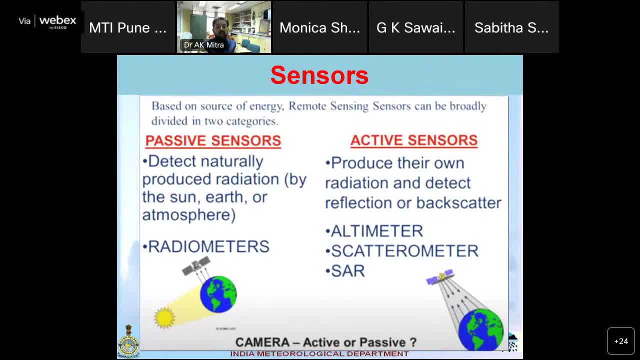 spatial resolution and they are very, very important for a particular kind of weather phenomena, particularly, if i can say, like radar, similarly sar, like synthetic aperture radar, basically the flood zone area or you can say the agriculture areas. they are based, mainly used for the active sensor, where the passive sensors are the basically based. 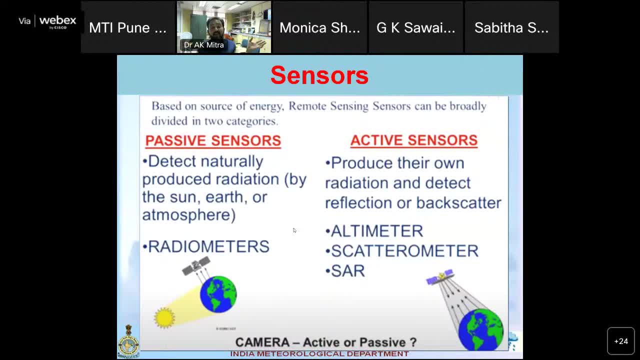 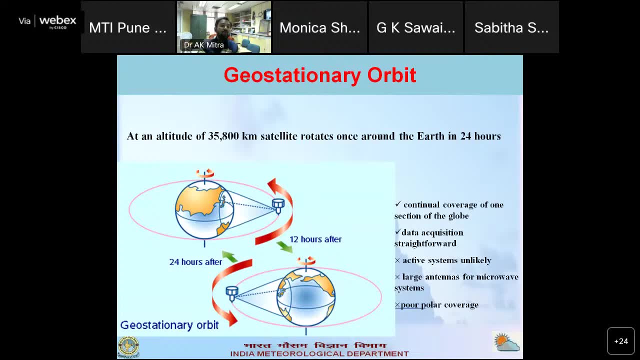 on the radiometers. so these radiometers give you the all information, what i just explained- thermal, visible and all kind of information. now, how this information could be employed to the satellite. then there will be a kind of a path where satellite moves on and that path is called. 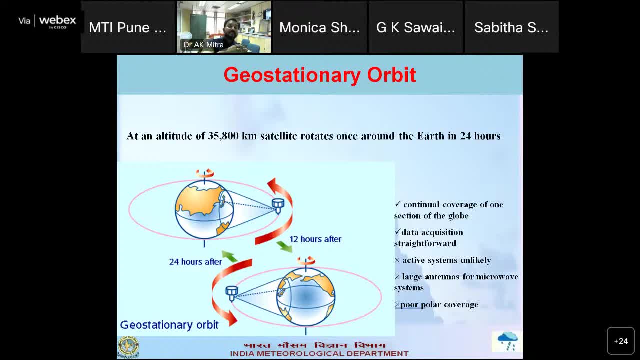 orbit. now here when we talk about geostationary orbit, that means it will be kept almost altitude of 35 000 kilometers, 35 to 36 000 kilometers, and that satellite rotate once around in the earth in 24 hours. so as image you can see it is rotating as according to the earth move its own. 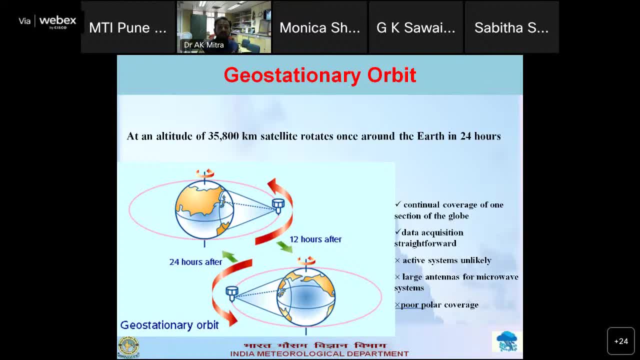 the moment of the your, the velocity of the satellite will be kept constant as compared to the earth rotating its own axis, so that what happened- continual coverage of the section of the globe- will be received. data acquisition straight forward, but there would be a very less likely of active system. large antennas or microwave system could not be possible and 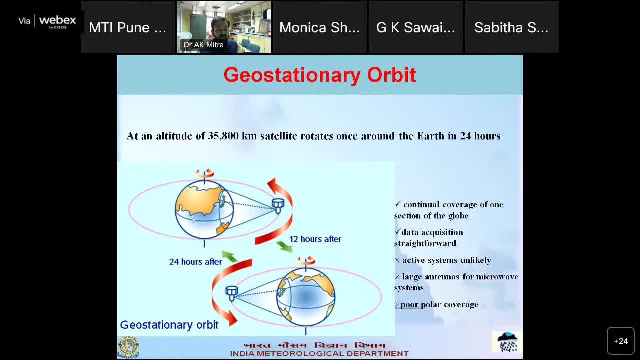 all the polar reason you can't get it. so here, 24 hour, you can get the information of your particular disk, as you know that we have a insect 3d, insert 3dr satellite. these two satellites are basically of geostationary satellites and then, second part comes, the polar orbit. so satellite. 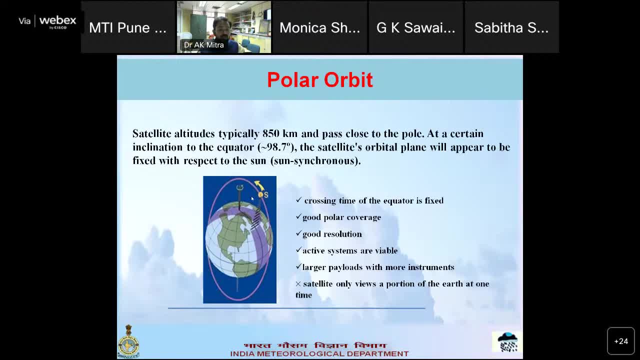 altitude, typically 850 kilometer, and pass close to the pole. as you can see the imagery it's: it is ascending and descending, it goes from north to south and south to north, and the equatorial inclination will be almost around 198.7 degree. so that what happened? the mostly information, you the 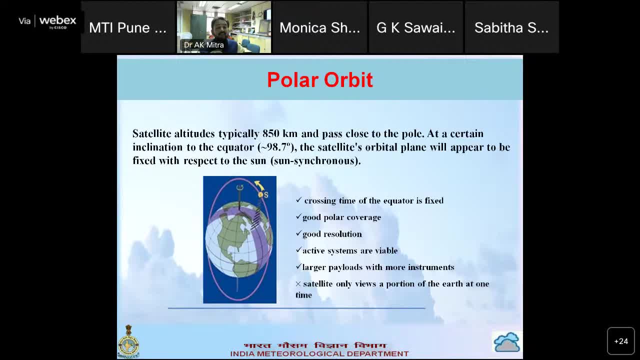 best information over the over the poles can be obtained because it is a sun synchronous in the geosynchronous. so the most important part is: crossing time of equator is fixed. good polar coverage, you can get it. good resolution, active system are viable. large payload with the more. 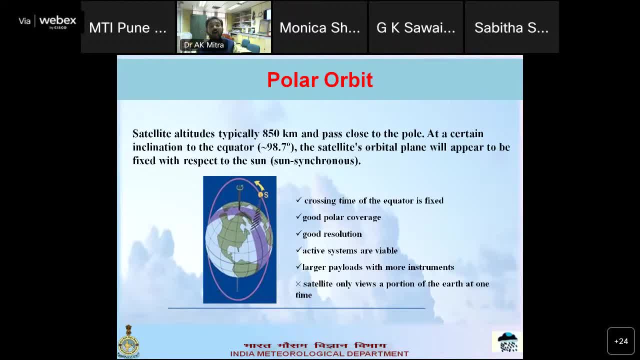 instrument. you can get it from here, but the only part is that you cannot get the continual coverage of the particular system. so, like you can see, uh, some of the events, like a cyclone, where you need to look at it every 15 minutes. there, your microwave could not play the. uh, you can say the. 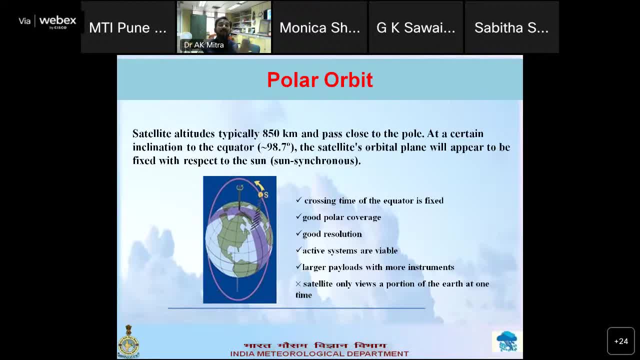 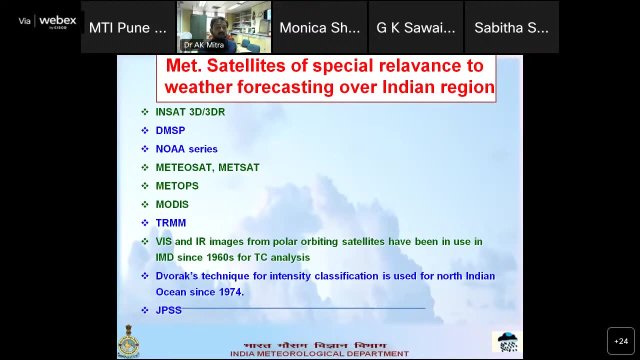 good temporal resolution. but here again the information. both have difficult, uh, different sort of, and they have a. both have their merits and demerit, but significance is more, uh better for the both these satellites, you can get it now. what are the mid satellite basically and where? what are the weather for use, for the weather forecasting you? 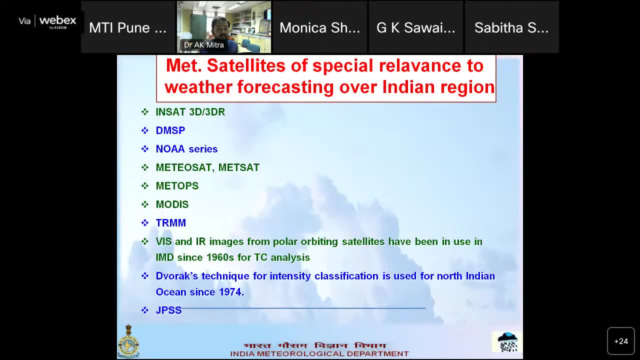 might we have that insert 3d, 3dr. we have then a defense um the msd dmsp. that is a noaa's uh, us satellite. noaa series of satellite. noaa started from seven, eight, nine and then it's eighteen, nineteen. now noah twenty, it is coming from jpss one. jpss two will come. 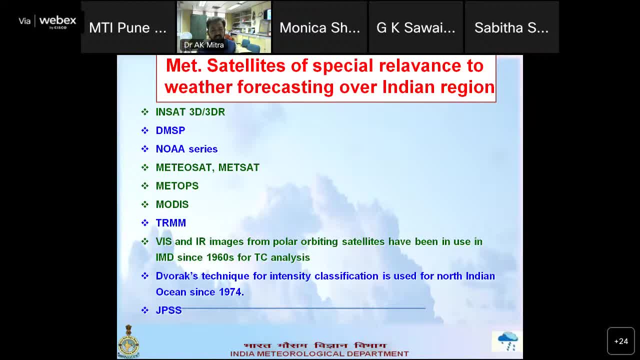 mother, metal and material set, that is european, and metal, then medsat, metops, that is european, uh, then mortis, trmm, visible and iron image from polar orbiting satellite that have been used in imdc since 1960 for topical analysis, so 1960 these these polar orbiting satellite have been used. 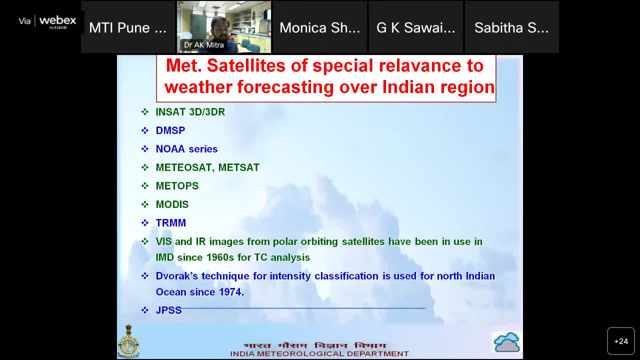 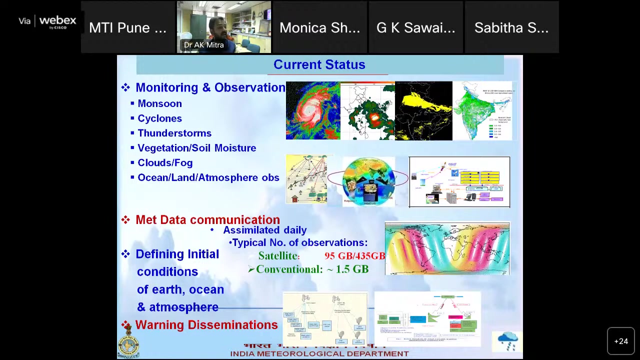 then devouro techniques for intensity classification for north indian ocean since 1974, and then jpss, that is a brain polar uh system, that is from the noaa no what 20. So basically these satellites have the main focus on that must be observations. So current status, if we can go by monitoring of the observation, like what are the kind of observation? monsoon, and you know that we are tracking the monsoon from the satellite. also cyclones, thunderstorm, 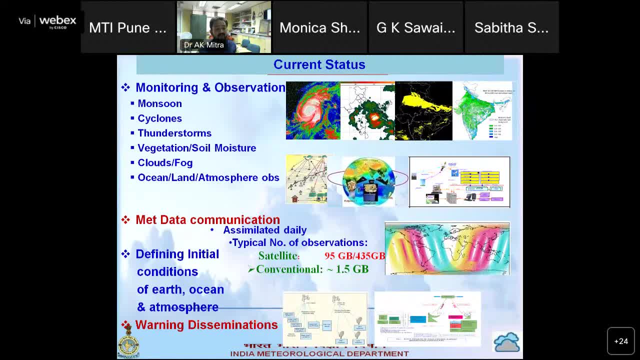 Vegetation, soil, moisture cloud for ocean, land, atmospheric observations and then make data communication. It is also going to the simulation cycle And there are the conventional image, that is, the satellite information. The huge satellite data is going to the uh model, a simulation. So, if you can see, there is a 90% of data being estimated to end up with the model. 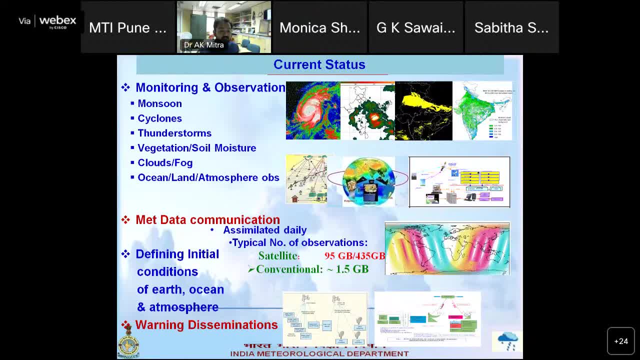 And and defining the initial condition of our ocean and atmosphere, and thereafter you can see, there is a warning dissemination. So these are the kind of a point where we are: we are disseminating this information to To the different sources like print media and stakeholders. 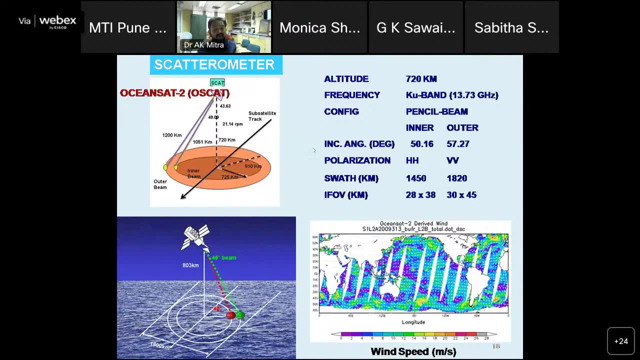 Scalpel meter here particularly just. I would like to mention that Here it is also kind of a polar scanning, uh geometry, where frequency is almost, altitude is 720 kilometer And polarization is horizontal and vertical both and similarly been speedy. We are getting these information on very, very information um. 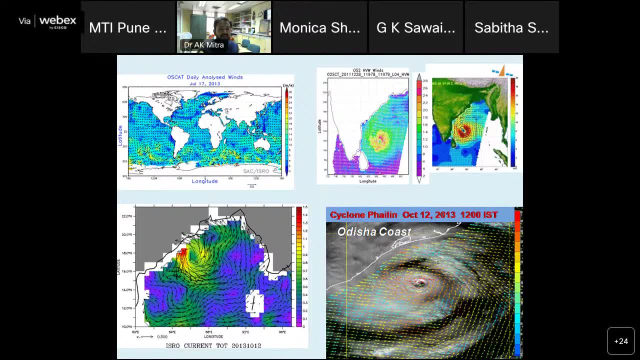 Informative, particularly for the any weather hazard. like Oscar twins you can see here, analysis wins And then, uh, this cycle failing. you can see: there is a, there is a, there is a bin, Or the, or the cyclone, it is a superimposed, or you can say it and computed. 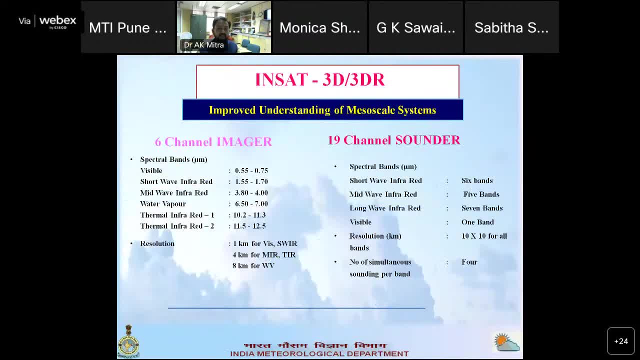 And and then we'll come to the our own Satellite insect city and, basically, as it is launched in 2013, for 13. And in the launch in 2016,. so there is a 6 channel image that we can see that visible short way via media. 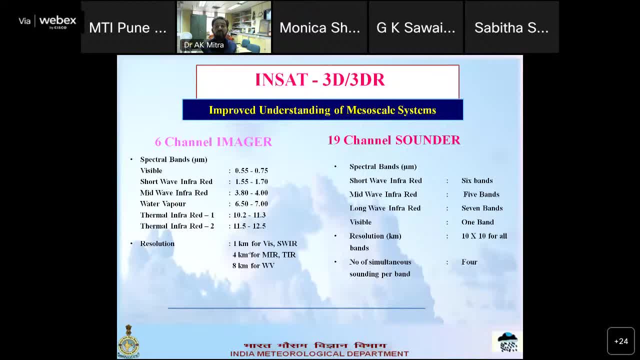 Water vapor resolution is also given resolution. Also, There is a paradigm shift in weather observation, particularly from because of This multispectral nature of the major 1 kilometer from visible as the blue wire, 4 kilometer for and 8 kilometer for water. 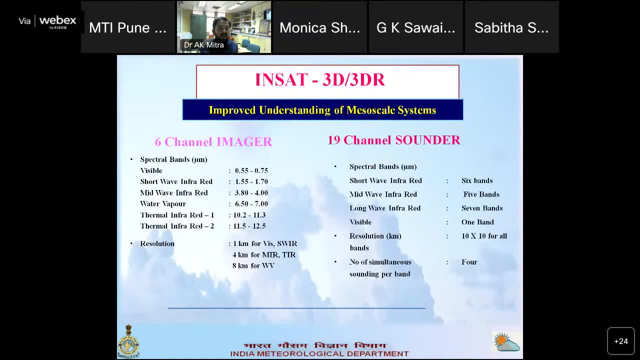 And and then the sound. that is also. it was 1 of the equipment um, which is uh, it, it, uh. it works like a radio. Sunday You can take the. You can say this could layer of the atmosphere by spectrum um, 19 channels of sounder. We are short way, medium, We have a long way. 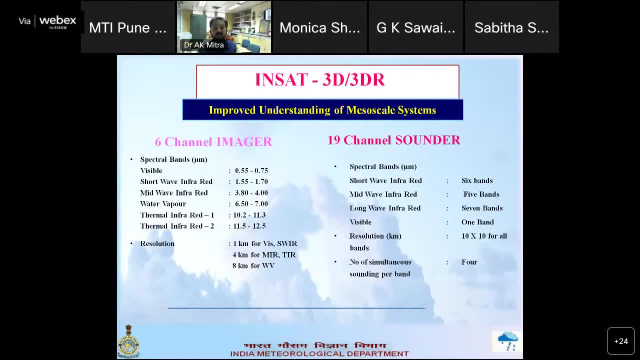 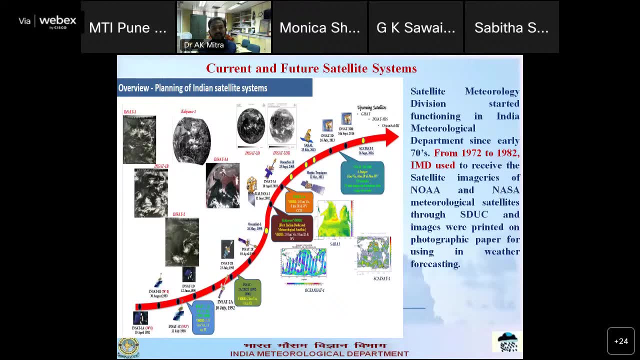 Uh, we'll be there. and there is almost 10 by 10 kilometer of resolutions. So, um, this is the current and future satellite system, that satellite metallurgy division. Uh, since early seventies- Yeah, That's So 1972 to 1982, I am the users to receive, as I mentioned, that, no matter that, NASA metrological 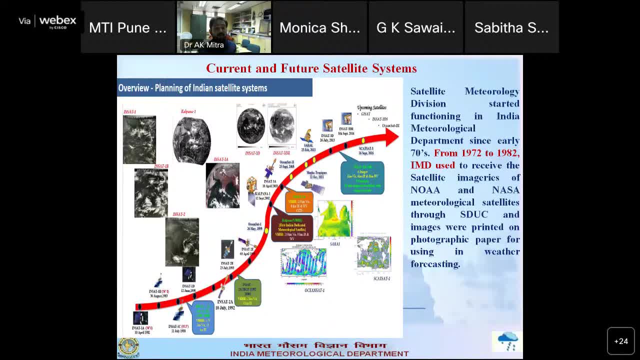 Through images were printed at that time on photographic paper for using in weather forecasting. You can see here, And then 1982, we have started in set 1 a series. Then 1 B, 1 D has come, and then instead to attend July 1992.. 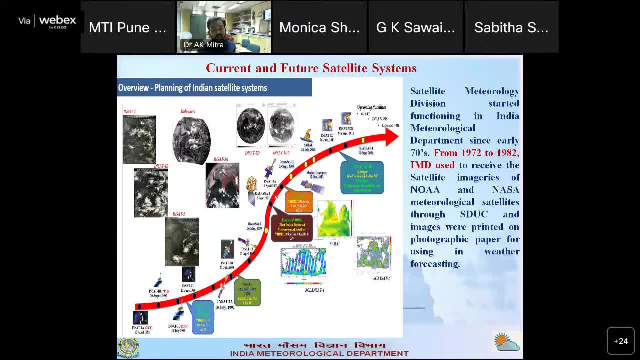 Instead to eat and ocean set. 1 has come and then calculate satellite. You all know that The famous astronaut that we named our satellite in the company, Then 1st Indian uh, your dedicated metallurgical satellite, where Uh resolution was 2 kilometer and resolution was 8 kilometer, and then 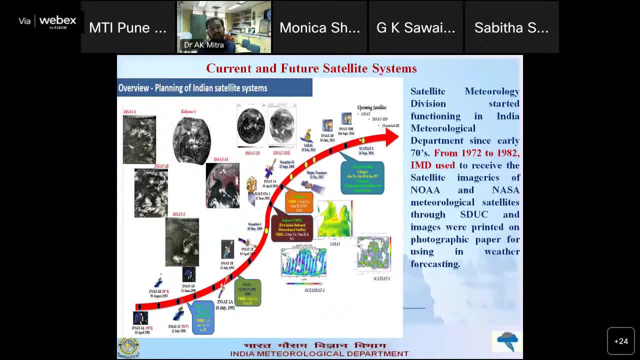 Instead of 2003,. ocean set 2, several instead of 3 D, 3 D R, and now he said 3 D S, and the upcoming satellites are also waiting for. So this is the full path of how satellite metallurgy division has evolved. 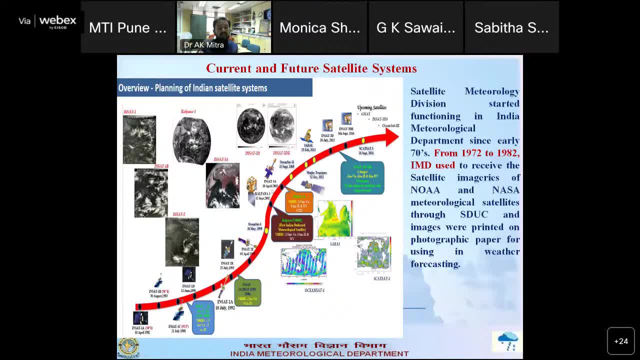 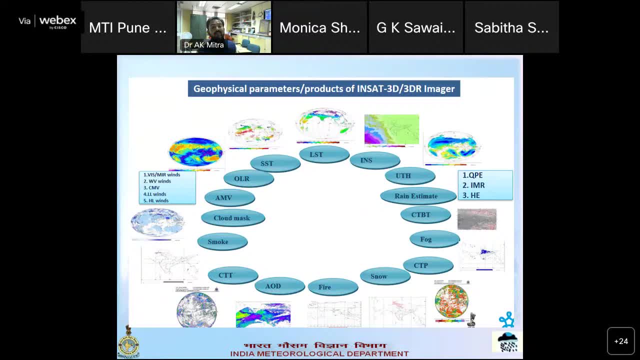 With a number of observations from different satellites since almost like 50 years Uh, and then a number of physical parameters, uh products from Uh you can see that that line service temperatures, the surface temperature, Cloud mass, more city, the cloud of temperature. 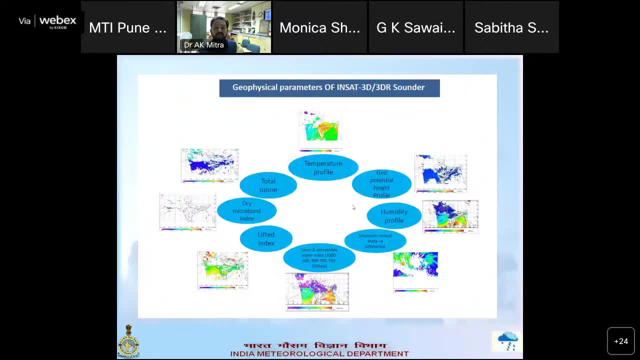 So number of observation has been has been received from these images. and then geophysical parameter of- instead From sounder like temperature profile, vertical profile- you can get it From almost 100 HPA, 50 HPA and total ozone lifted index. humidity profile, your potential life. 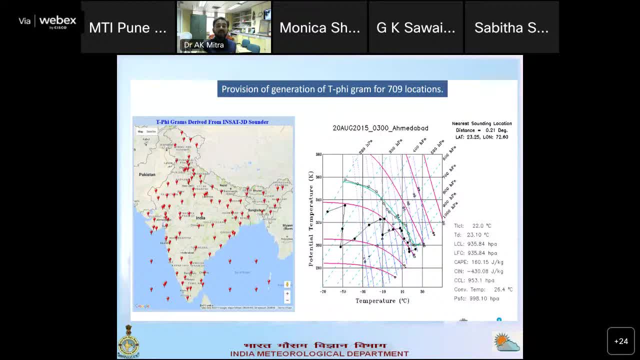 And this is a T 5 gram which is most useful for Sounder data. you can, you can receive it and then you will get it all. the, your conviction, uh, convicted, temperature Charge couple, you can say the- and LFC, low compensation level, that that kind of information. 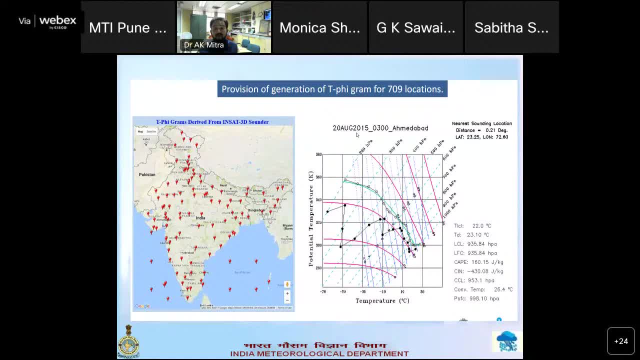 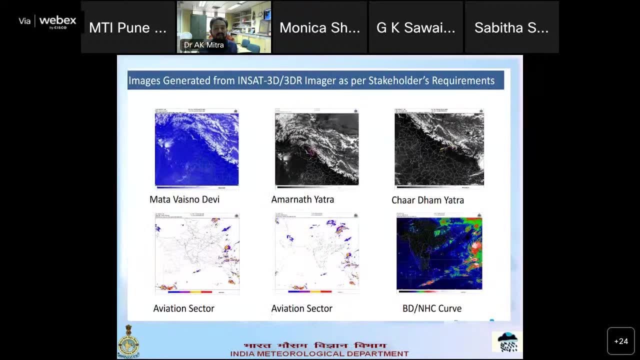 Which is most crucial for the weather, to see the convert to whether that information also been derived in terms of- And these are the images generated from- instead of stakeholders, like you might have heard that my, my, uh, my, you know maybe. 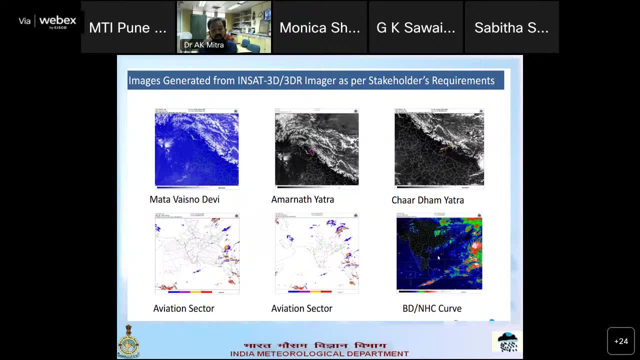 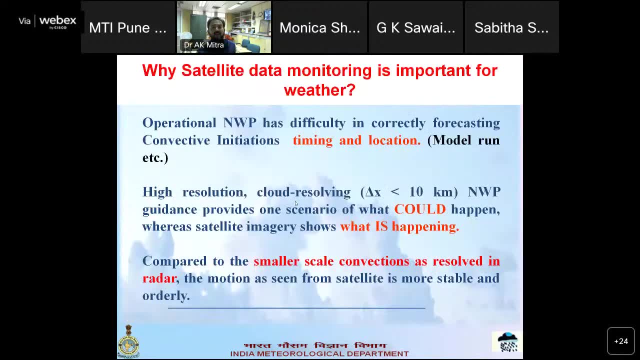 I'm not the other chart on your aviation sector. And then so number of observations also taking, and we are providing to the different stakeholders. No, the importance of satellite metallurgy, or you can say satellite remote sensor, or you can say 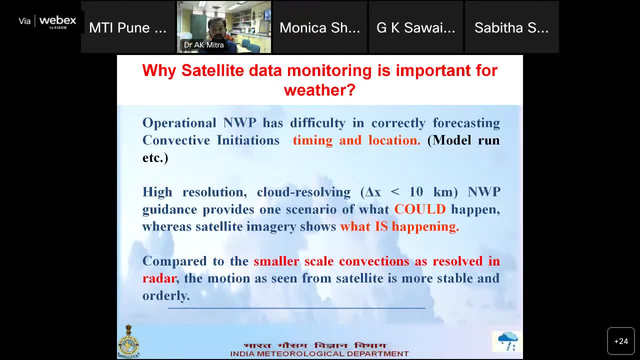 How it could be used. the most important thing is that weather enemy, weather forecast. now in weather forecast it comes that That immediate now cause. the most important part is how I operational. you know that if there is a, there is a uh kind of difficulties in timing and location because of the model. 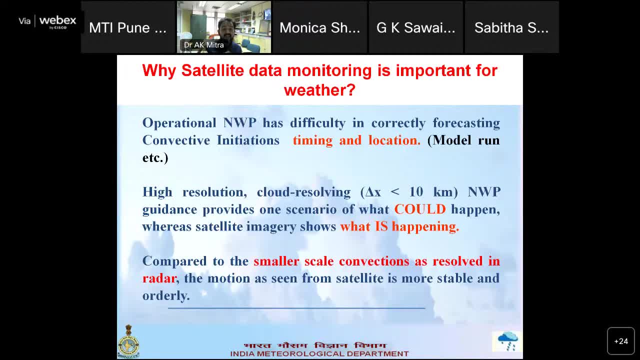 But here, uh, and then model, I will give you the what could happen, but your satellite will give you what is happening, the current status, and with the play of animation you can able to see what is Happening. that now casting is most important part of remote sensing from the weather forecasting and a smaller scale of conviction has resolved in the radar, as we can see. 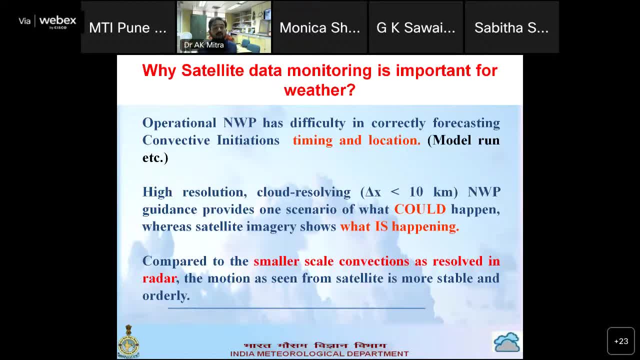 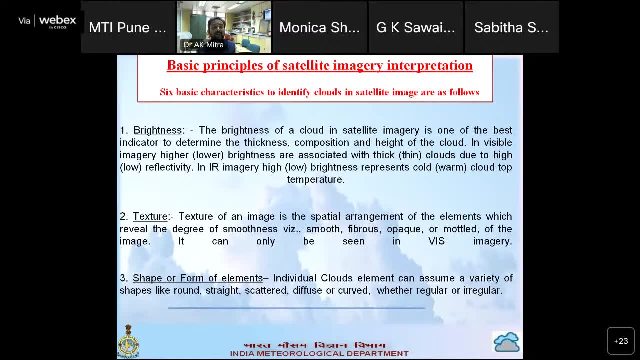 The motion you can see in the satellite or animation is more stable and orderly. Find out to detect the weather phenomena now. now it comes to the kind of a how satellite immediately could be interpreted. So there are 6 basic characteristics To identify cloud in satellite images like brightness, texture, shape of form, elements. 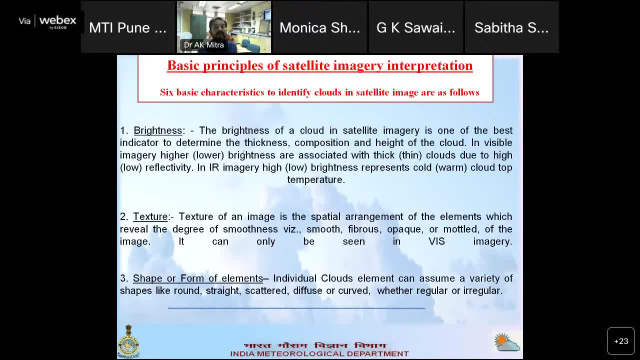 So brightness in the cloud in imagery is 1 of the best indicator to determine the thickness, Composition and height of the cloud. invisible imagery brightness are associated with the thick cloud due to the high reflectivity In either imagery brightness in present the cold, that is, a warm cloud top temperature. So these are the kind of information that you need to look at. Then, 2nd part, is a texture shape of the uh. 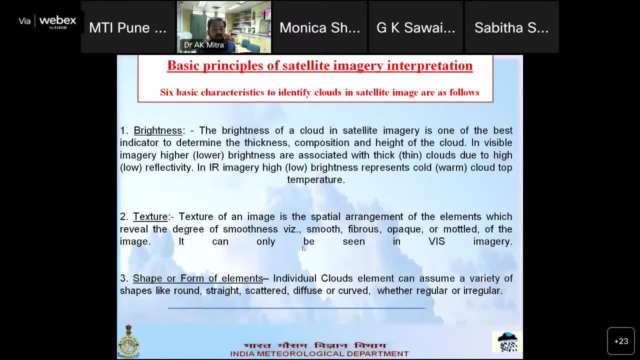 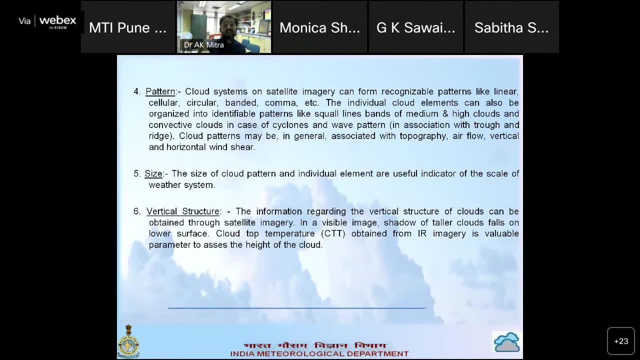 Uh, elements. what kind of shape this particular cloud is having. I'll show you the example And then pattern. how cloud system on satellite imagery can be recognizable, like whether it is a cellular or circular, Blah bandaid comma. how it is then side. what could be the cloud pattern size. 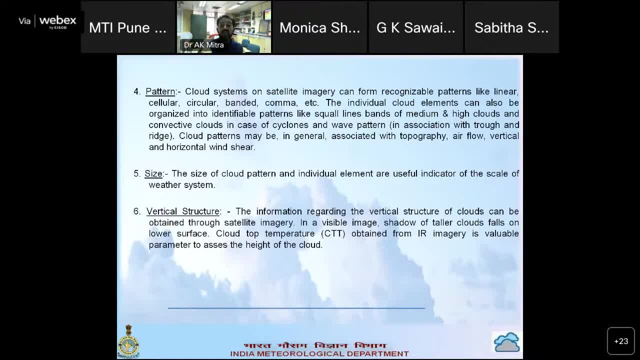 And where, where, where the element are useful indicator of scale of other systems. a monsoon is a huge extent, So that is a site, very important matter here, But if the thunderstorm, it will be very, very small scale. A cumulus cloud, similarly vertical structure. the information regarding the vertical structure of the cloud can be obtained through satellite imagery and then CTD. that what I wanted to say. the cloud top temperature is obtained from imagery is valuable parameter to assess the height of the club. 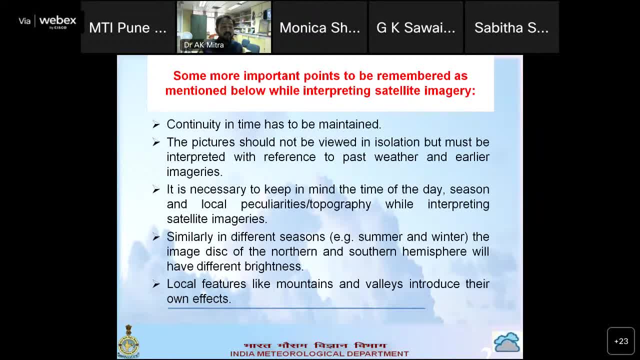 Now, some of the point that we need to be remember, and that is the most important, is by seeing from the geostation, the satellite, that is, a continuity in time has to be maintained, and then the picture should not be viewed in isolation, but must be interpreted with the reference to past weather and earlier. 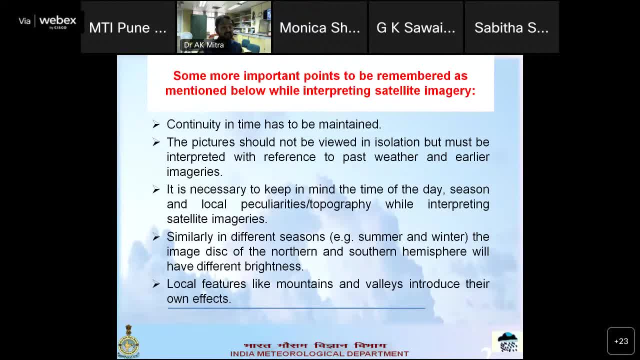 And it is also necessary to keep in mind that time of day, season, local peculiarities, topography, while interpreting satellite images, So like if you are seeing the summer or winter, and now what kind of northern and southern hemisphere will look like, that brightness will make changes. So this also also kept in your mind. and then local features, like mountains. 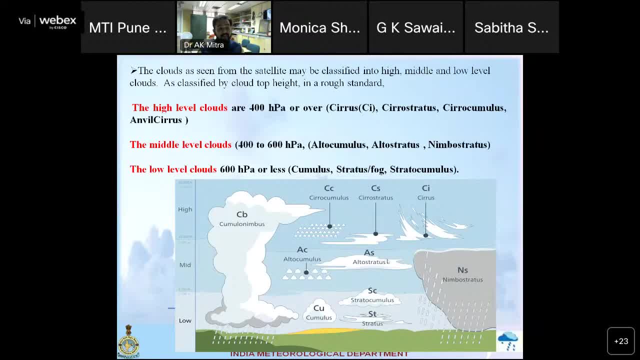 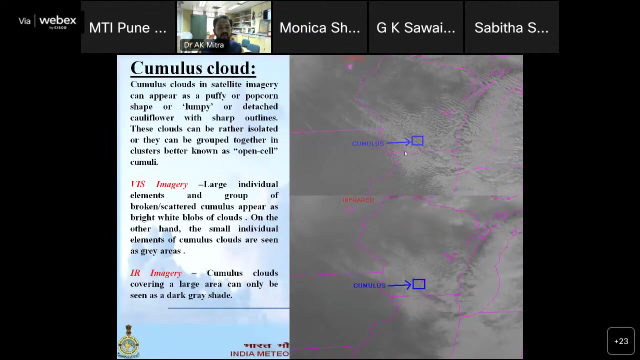 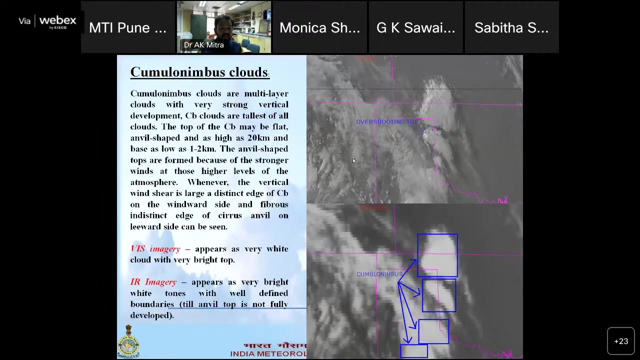 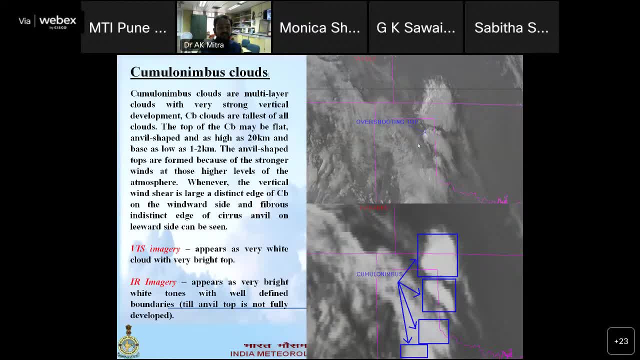 white club You can see here. This white image is this patch in this is a Atlas, whereas very imagery It appears very bright white tones with the well define boundaries that you can see in. I I did So. in that way I am visible. both can be able to detect about CB and let me tell you this is the very important for the 3 months. will see then. 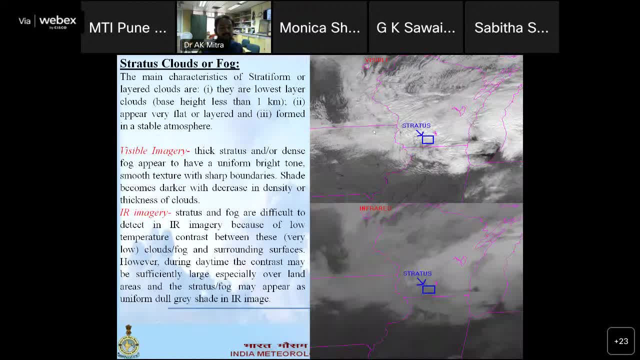 Then status cloud in a visible imagery we'll find out. the thick status or dense fog appears to a uniform bright tones. They have uniform by phones but with the imagery because of the lower temperature um the cloud fog surrounding during the daytime contrast maybe sufficient large, especially, especially over the land. 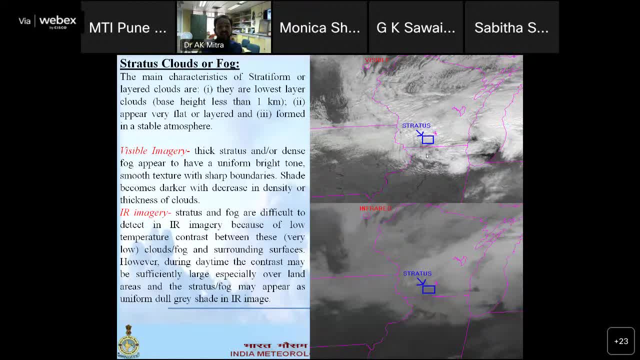 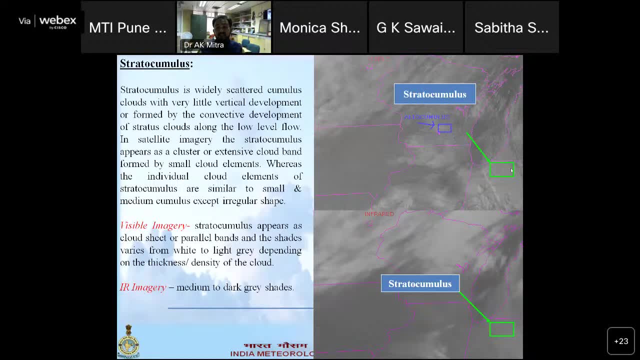 So here status will be: look like I am like this and set us like this and then start a common loss that we have seen a set of visible imagery appear as a cloud sheet You can see. these are the sheets: complete um, uh, low BT of sheets and parallel bands and shifts where the I are medium to dark ratio. that you can see: medium to dark ratio. 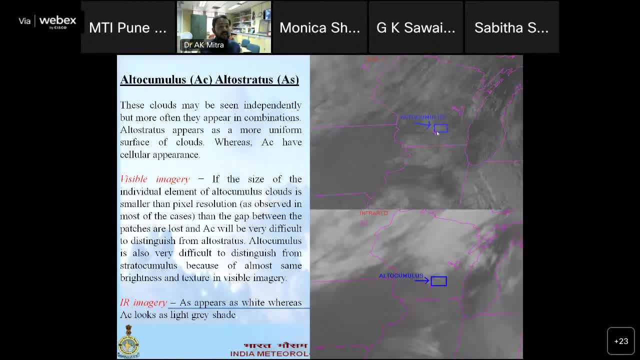 And now to cumulus. similarly, the size of the cloud, if you can see uh individual element all to cumulus is smaller than the pixel resolution: Very small cloud. Similarly, for our imagery it appear as a look like a gracious, like you can see here. 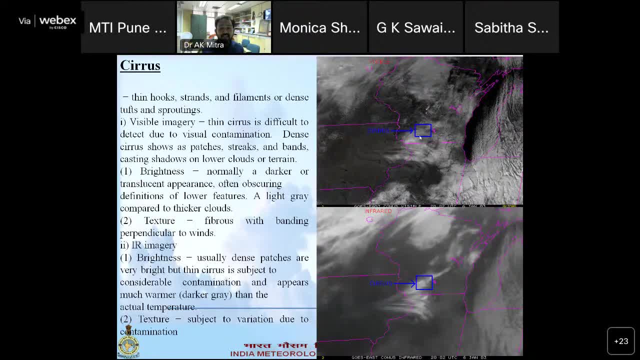 Similarly the serious cloud series. they have a different structure. You can see in the series Things it has is difficult to do: Detect, because the resolution is to be a 8 kilometer. It is very difficult sometimes but then it shows that the patches that you can see here, whereas in the brightness, uh, you can go by. 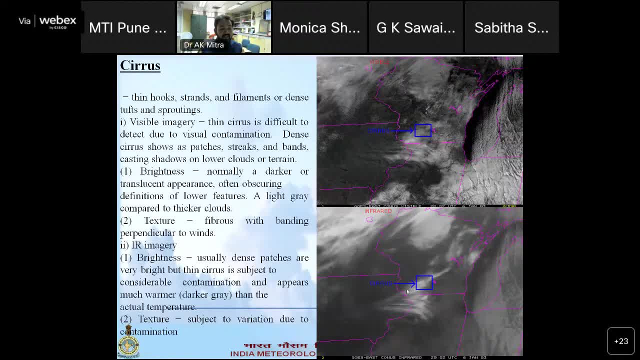 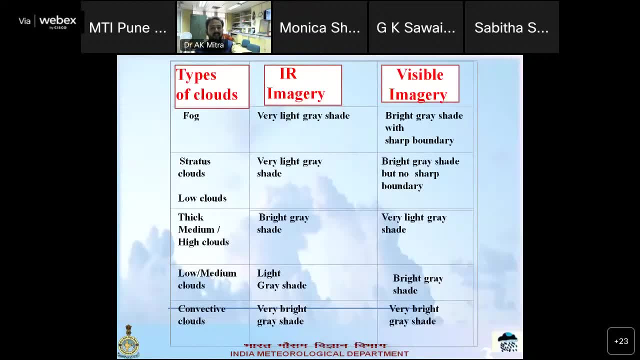 I are very bright, but things that are subject to considerable contamination of much more. This is the darker That you can see here. so so this is the 1 table. that uh what I have explained that. how far could we look like? and I are invisible, like very light ratio. 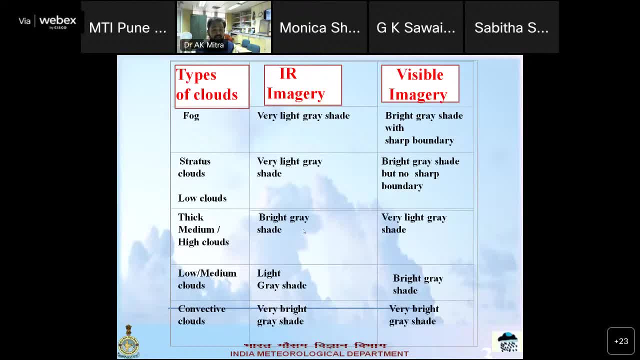 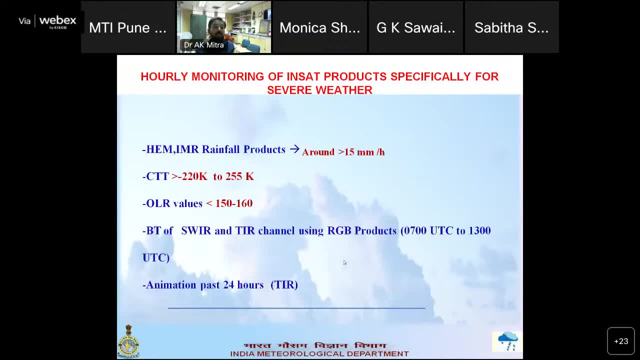 Similarly status: cloud: very light gray. thick. medium high cloud. bright gray shades. Very light creation. low medium clouds. very bright extension. So these are the most important parameters that you need to, most important features that we need to look at, and then some of the products like- uh, I do estimate This is the rainfall products. 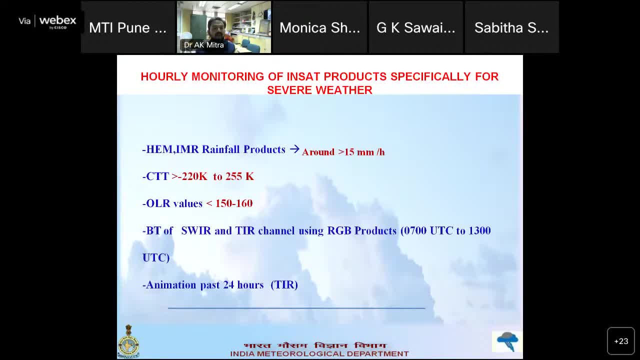 Uh, multi, um, you can say the multispectral rainfall, So some threshold, like if it goes more than 15 million, you can around, you can say that it is the more we're going for Cd. if it is going more than 220 to 255, that means there is a conviction. 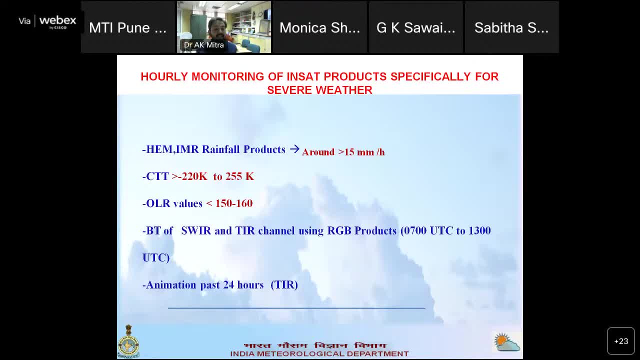 Well, our values, If it is less than 150, then there is a conviction. Then the RGB that I will come to the uh, I'll show you the imagery, then you will be able to understand, and then, finally, the animation. 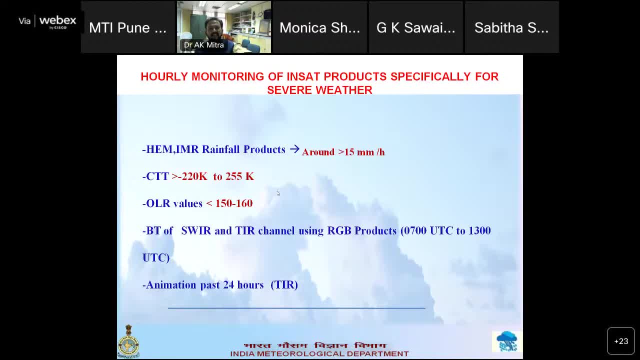 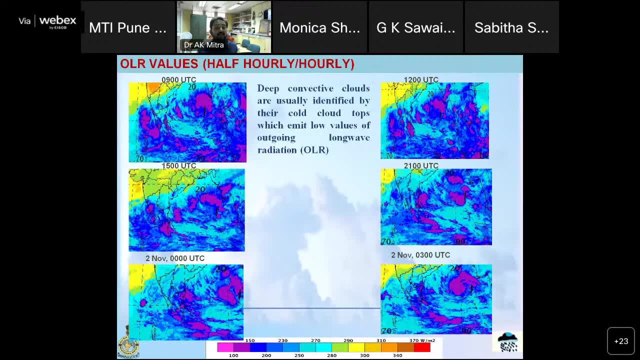 So these are the 4, 5. in the broad window you can see if we can go with the satellite image and by this concept you'll be able to better way to see the Natural weather. like you can see the deep connect to cloud. If you can see if it is less than 150 to 160, this image low value about going radiation. You can see here This. 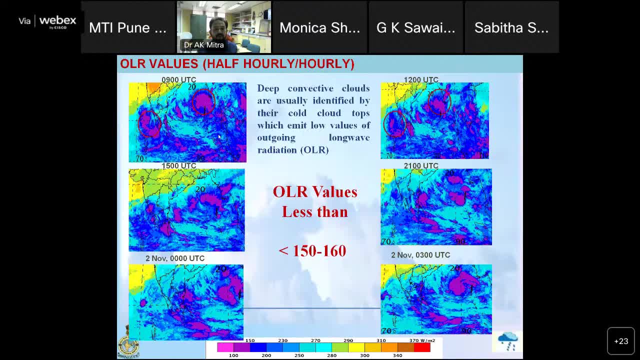 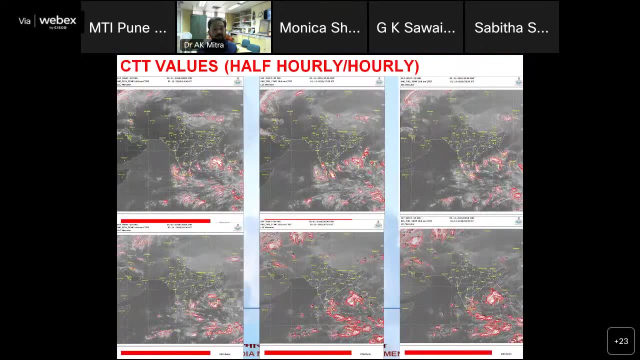 This part. They are the very, very, very low. Uh, you can say: well, our value, deep, convicted clouds are Can be seen from this window. that is less than 150 to 160.. Now you can see here like this: so these are the, and then, similarly, that is a cloud top temperature. You can see here, cloud top temperature will be look like this: 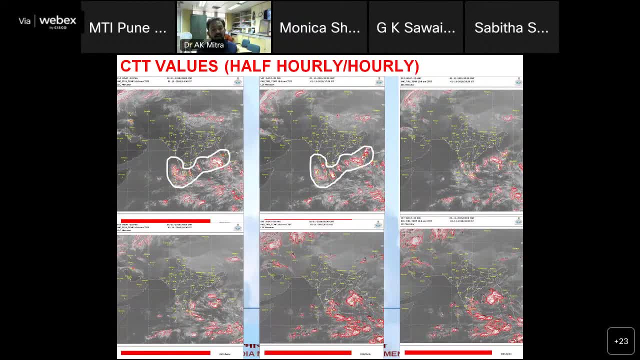 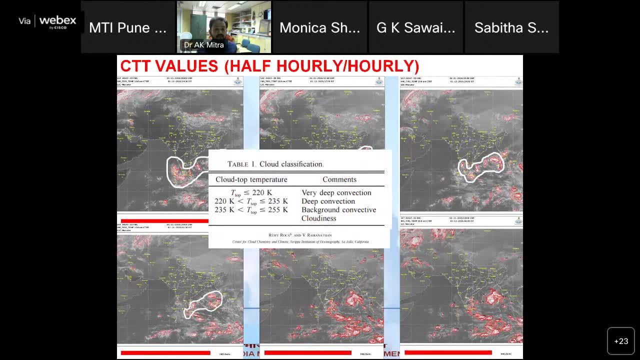 So so like on the 1 to you are almost luxury area, The huge cloud top control. you can see and you can. you can analyze it. So like a very deep convicted Now less than 220. most important here, that how you'll be identifying the deep convict people out to 20 to 235.. 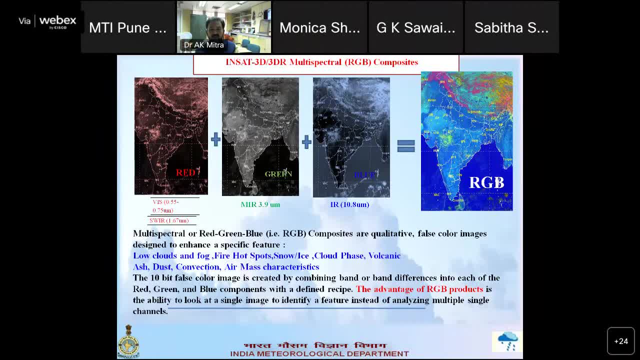 Background, convicted flow to 35. and then the new thing that's come, that is the RGB and the most important and more successful Uh worldwide, that detecting the weather from geostationary platform using the red, green, blue composite. Basically it is nothing, but it's the multi spectrum composite qualitatively false color image. 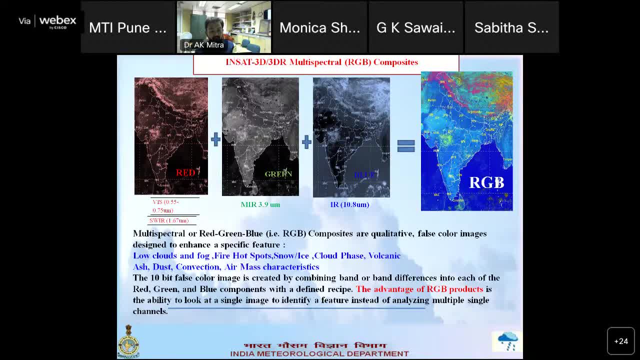 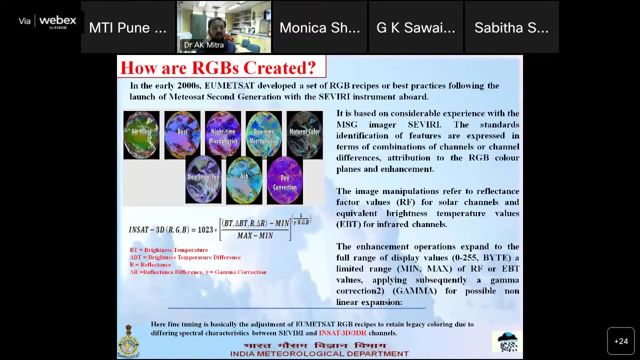 The design to enhance the specific features of local Cloud face, volcanic, as does convection air mask, Don merchandise. so the advantage of these major is that because all these are visible, I R, I are all packed into the 1 rgb image. Like you can see here, it has all started from in a year 2,000, by humans that they developed this RGB and we brought it in it And we put on introductory thread. 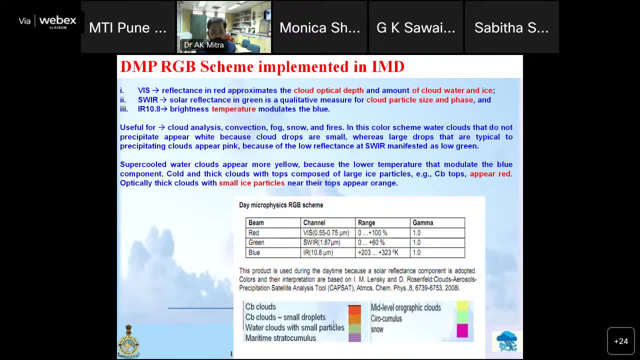 I'm because we can multiple features, like you can see the The top column. your seeming cloud look like it does a color code that you need to understand. like cb cloud will be like brick color cb cloud: small droplets and then water clouds, maritime cytocumulus, no, zero cumulus, mid-opera orographic clouds. so they have a nature of like. 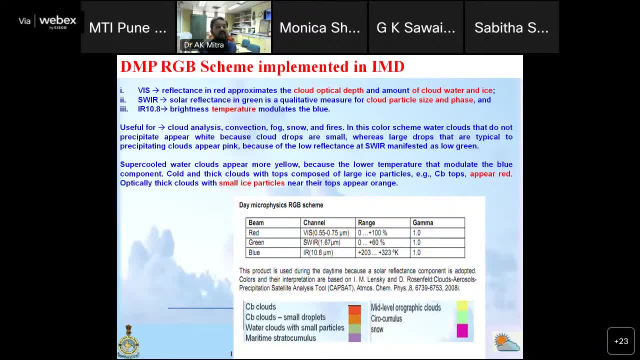 how they will see like visible, will see the reflectance in cloud optical depth and then swl will see the cloud particle size. these are too important when they merge and then ir modulate the temperature color. that is the blue. so then, when they color like put, 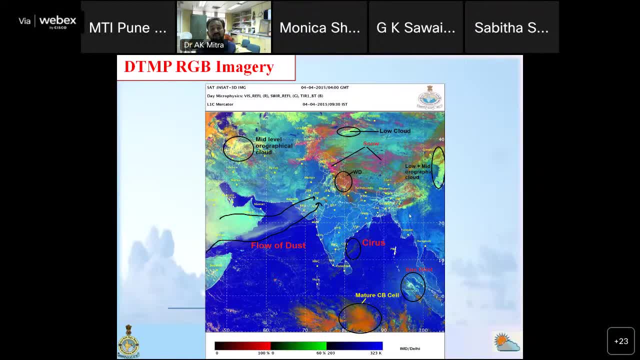 layer put into the one one image, you can see the multiple observation. you can give multiple events that can be seen by the only one image, like mid-orographic cloud over over over this area, then western disturbance, snow, low cloud, flow of dust, cedars, sun glint- many features you can see. 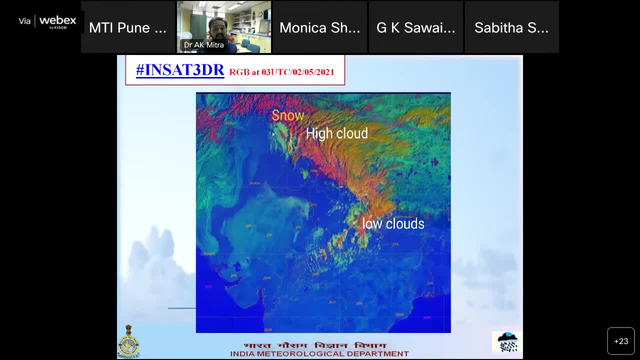 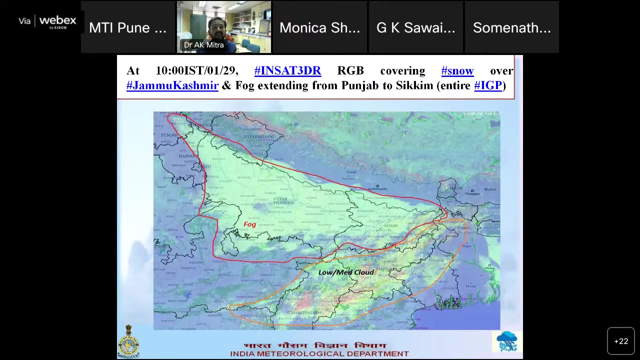 by only one imagery now, like you can see the insert 3dr imagery, like snow, high clouds, low clouds, by seeing only by the color code only you can able to understand how the snow is being forming and where the snow is being there. high cloud is there and low cloud is there. and then insert 3d rgb are also covering the large extent of fog. 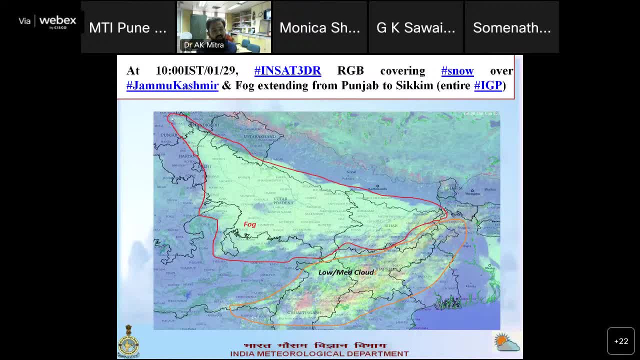 that you can see from our rapid that right from here. you can see here from punjab to almost like seeking around west bengal and near the banglades and then this: but whereas if you can see the lower pattern, lower bound, you will be finding out low medium cloud, upper part is the fog, so this. 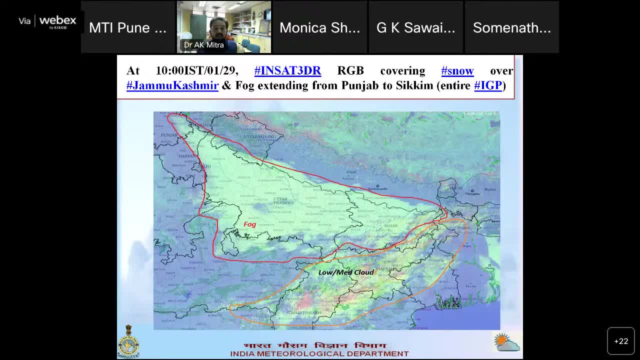 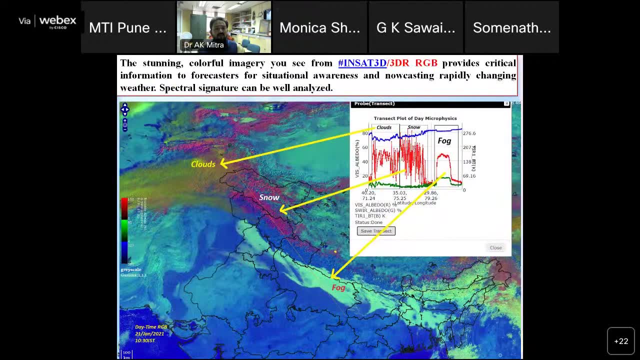 extending or delineation of fog and low medium cloud is very much important and this rgb help us to do so. like that. these are the stunning colorful. is this imagery, what you are looking at? this information very important for the forecaster, for situational awareness and for the now casting, because this spectral signature 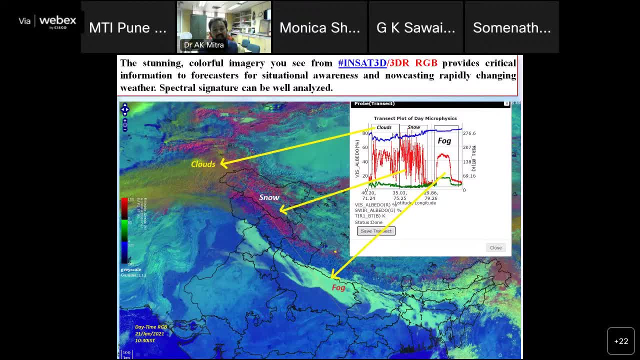 can be well analyzed, like: where is the cloud? the cloud, if you can see, like here, temperature is very less, where the snow, you'll be finding out- there is, absorption is very much, and where the fog, but the reflection is the most place, the important mode. so three phenomena can be seen from from this. 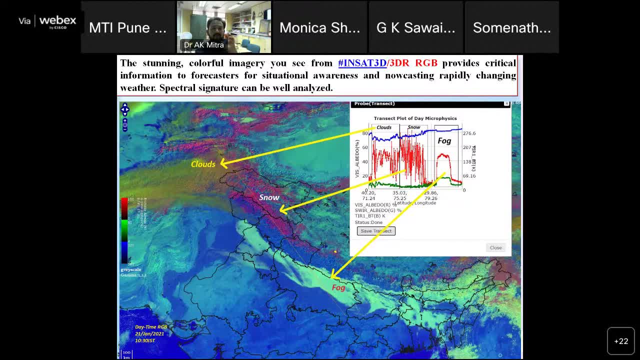 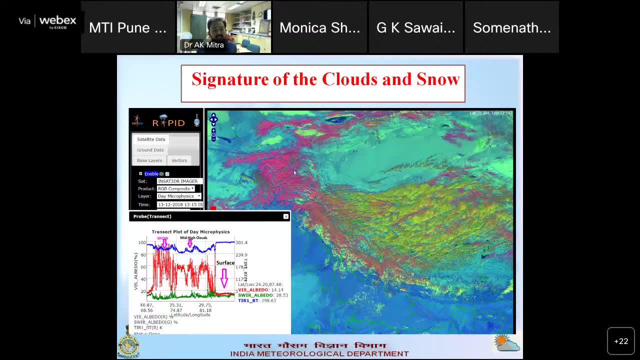 3d, 3d rrgb. that is a very spectacular image, or you can say the imagery, depicting all kind of clouds, snow and fog and then signature of cloud and snow that can be seen over the jnk. from jnk to you can come to the nepal and not that area. where is the snow, where is the mid cloud, where the surface? so 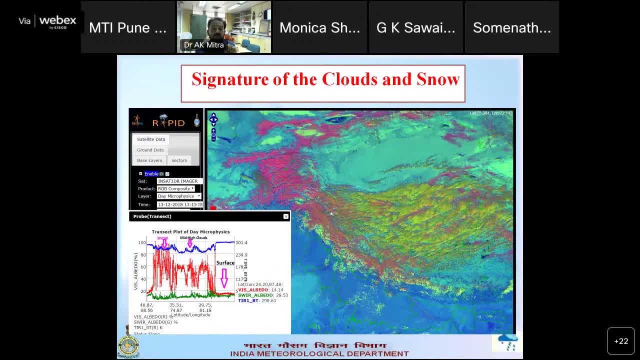 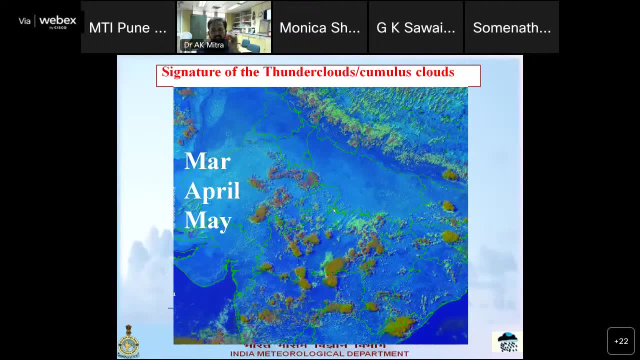 these, these values could give you, these rgb values could give you to help you to delineate this weather and then thunderstorm, thunderstorm or thunder cloud, cumulus cloud. this is march, april, may. you can find out small, small, that small pixel. that is the cumulus, that you can see, that, and 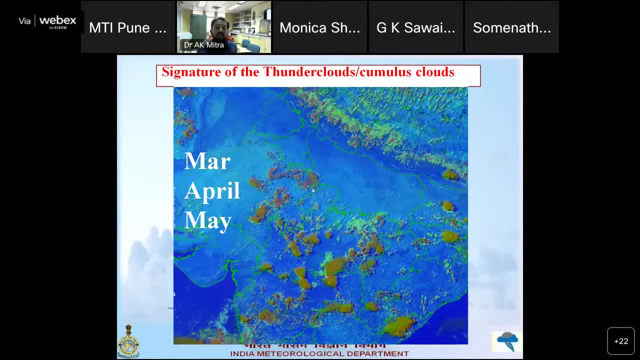 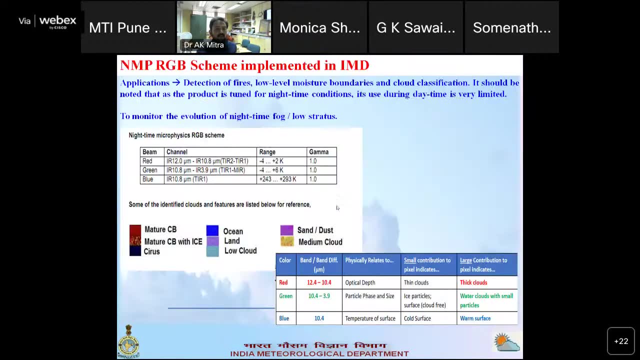 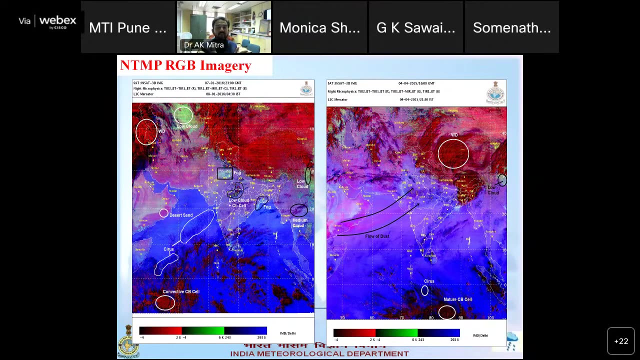 then whatever this brick color, what you are finding, this is a mature, that is, a thunderstorm might happen. thunder, thunder, cloud water, liquid liquid water content, all these things are available, so so, similarly, nighttime, also rgb. because we do not have a same channel, what severity is having, so we fix it to the different color shape. so in the nighttime these rgb will. 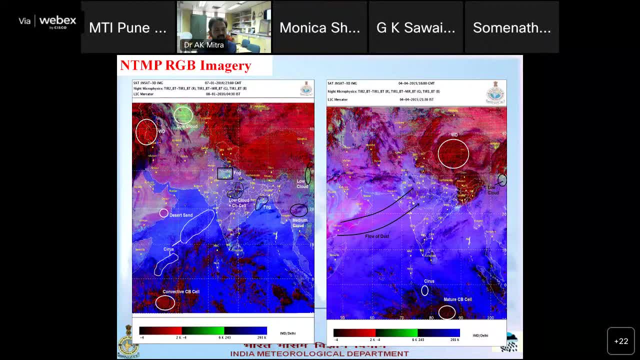 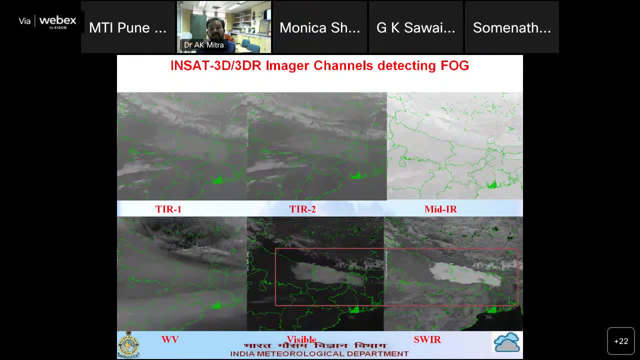 look like this flow of dust will be lacking, like this western disturbance, low cloud and this feature. so daytime and night time both play. they're very important. like you can see, tir2 and swir fog can be seen very well where the tir1, tir2 media here, whatever, you can't find the 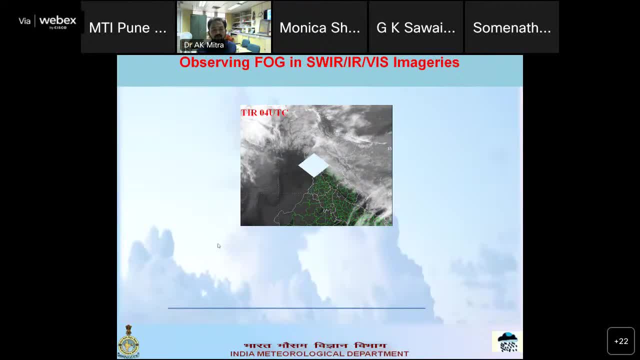 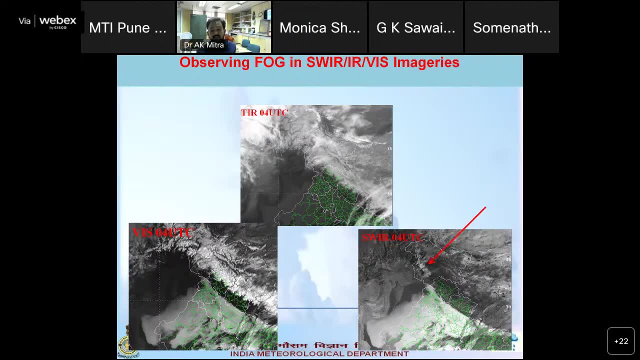 this fog ring. one more example i'll give you like, like you can see what the jnk and you will be finding out there is there is a swir visible, an ir channel you'll be finding out there in the srinagar there is a kind of a fog and which can be helped to detect it. like you can see here, this is the fog. 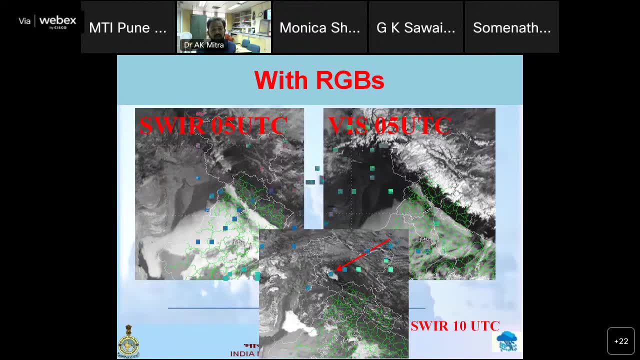 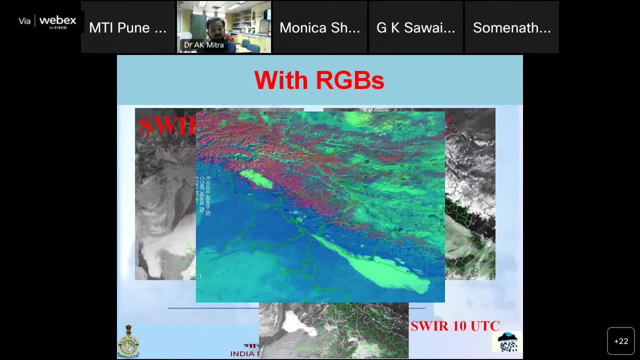 that can over the scene of the valley, entire it has been covered, whereas then rgb, it is clearly look like where is the snow and this is the your fog, and then this is like this one. so so this this has helped us a lot, like daytime fog. how you can detect it. this is the one parameter, that is all. 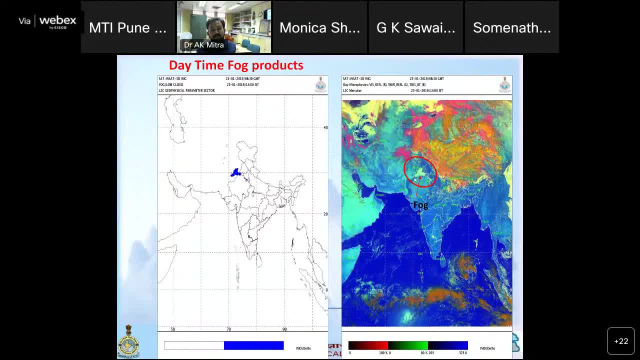 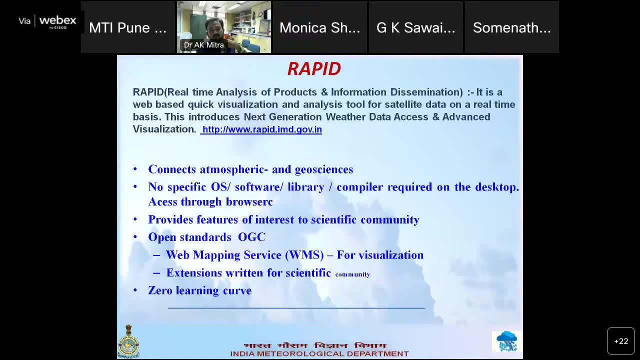 product that's fog local out, and this is the rgb. exactly that shape has been captured from the. so daytime, nighttime this fog area can be seen, and then rapid. as i mentioned, that the tool. i think everybody should go to the, this rapid tool where they can analyze by own. 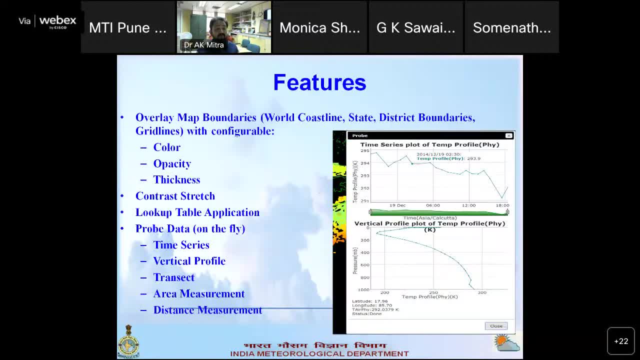 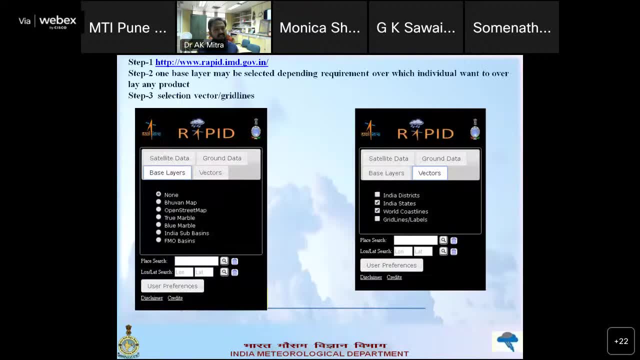 you can see that features that can be analyzed- color, opacity, thickness, time series. you can plot transit area measurement, distance measurement that you can be seen, and then open street map. all the maps are there. it is a well uh, self-explanatory. you can click on this and other ways you can go to the website: our. 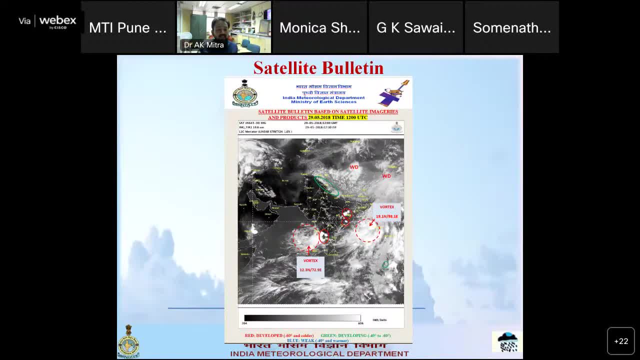 document is, report is also there. and then, finally, we are also putting the satellite bulletins every every every three hour, three hourly, and sometimes it is hourly, and with the, with the help of satellite data. where the vortex is, where the wd, where is the? your observations are so this: 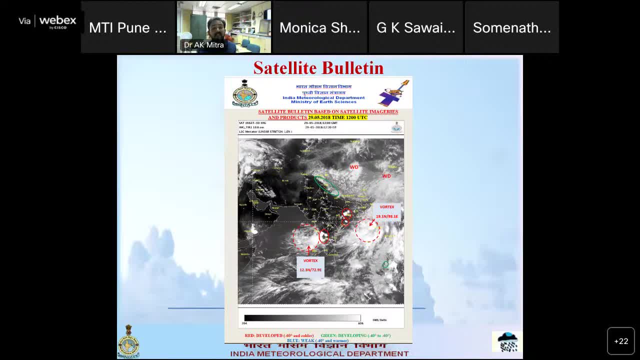 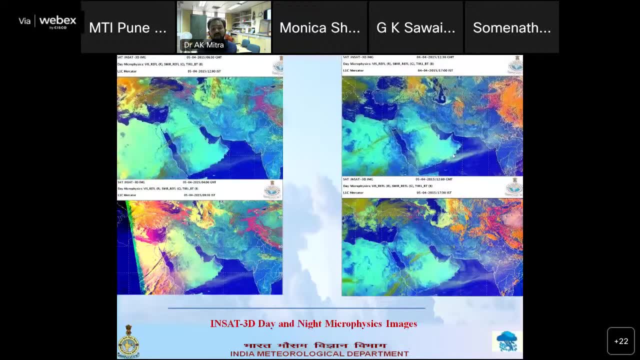 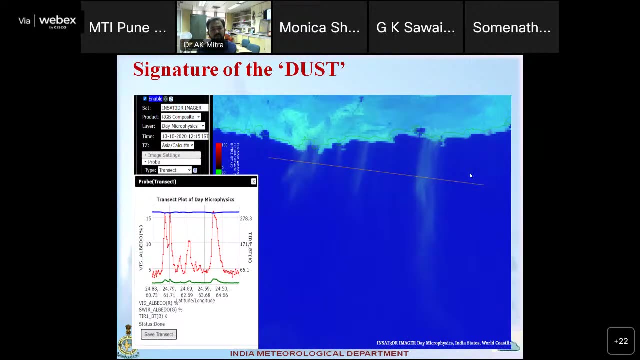 developed um and developing and weak. these three conditions are also putting into the our everyday satellite bulletin some rapid cases like: if i can, you can see here I can get dust. this dust is flowing from the arabia to the northwest india. they are mainly affecting it, like you can see for this pretty, very finer detection of the dust. 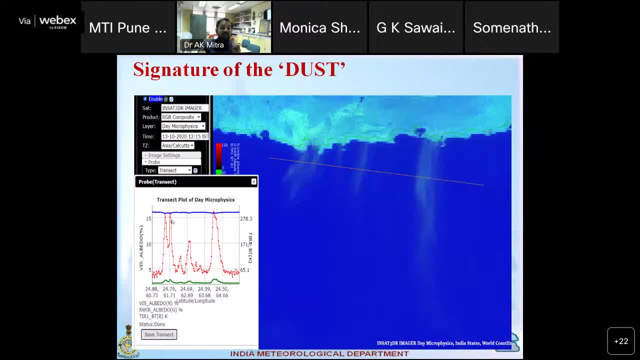 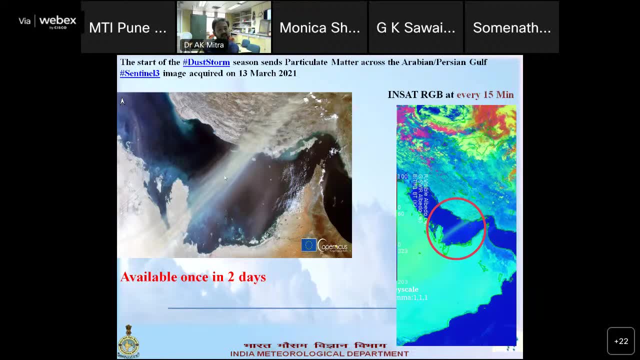 by the point also, by the values also, you can able to delineate where the signature of dust can be found. now you can see here: the dust storm can be seen over the centella imageries very sharply. you can see when you insert 3d or satellite images also you can 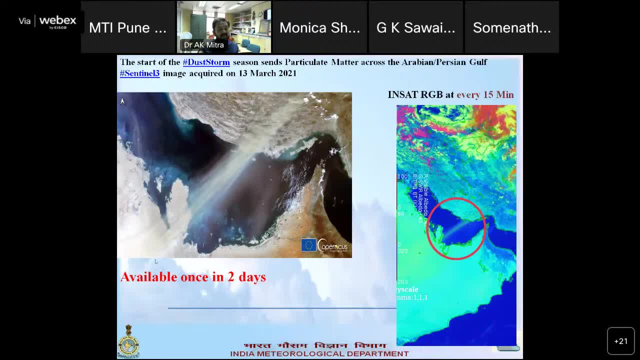 get it. the most important part is here that central imagery you will be getting every two days, whereas getting every 15 minutes. so that that's the most important, um, you can say, the tool which a forecaster can utilize, because two days waiting for two days that we can go for every 15 minutes. 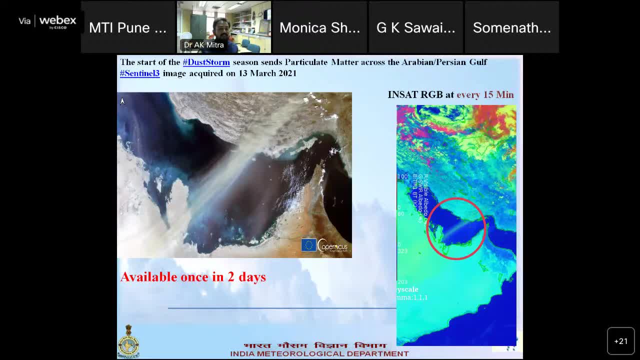 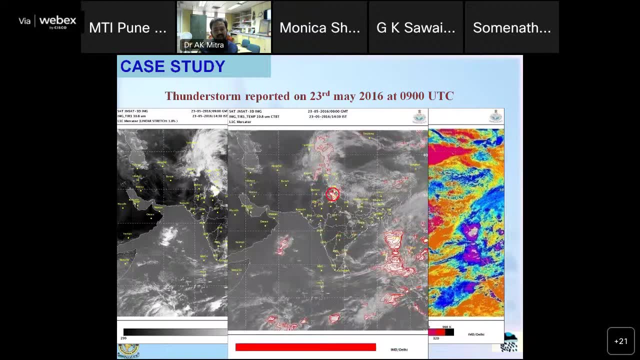 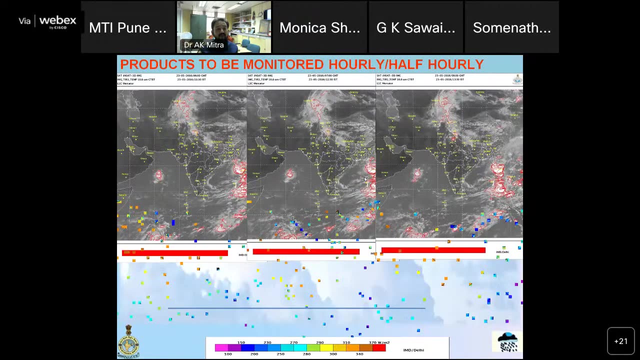 and that could help us to help us our forecast distribution. and now this is a thunderstorm. we can see here over the daily this reason. you can see the high ctt values. you can see by ctt values, you can, you can detect it. and then this garden daily reason and if we can see here, if i click, 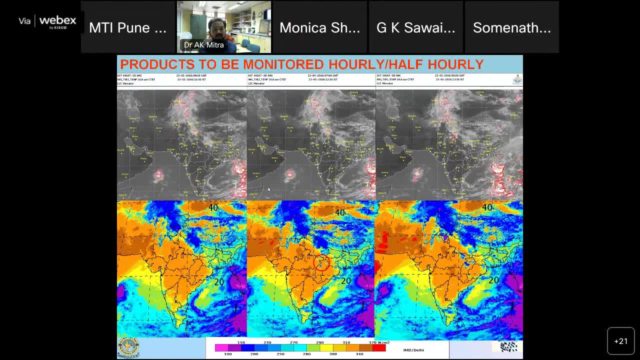 on, then you'll finding out the uh well, um denoted the values you can see. tt values can be seen like you can say daily, and chutney's got small parameter oil and, as i mentioned, the deep convective cloud of the 150 to 160 can be very well diminuting this kind of, you can say, thunderstorm. 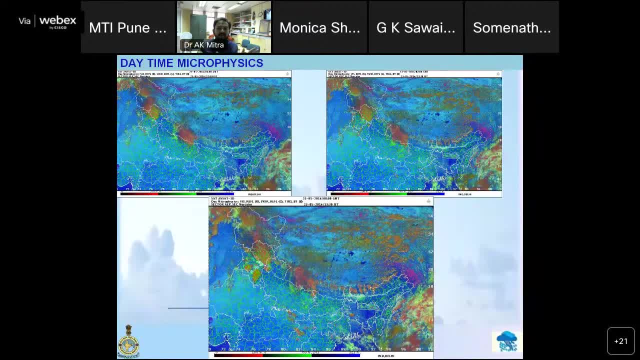 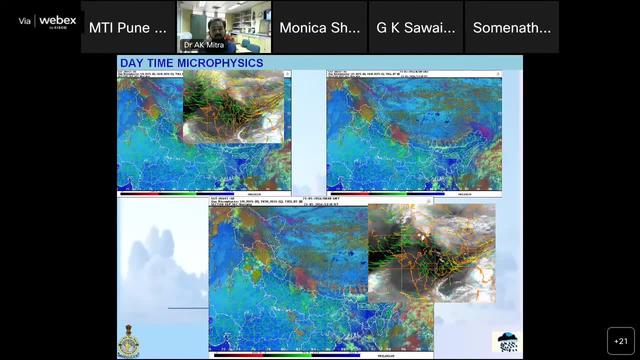 activities and then rgb. so there are many parameters are there. you can choose any one of them for you. and if you would like to go for the desert, like daytime, um, micro physics, that is rgb- you can take the wind. wind parameter can also be seen, uh, and then you can calculate and you'll finding out. you. 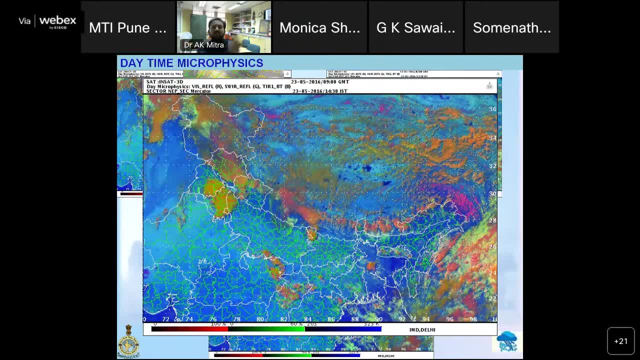 see, these are the daily reason. and chutney's got brick color. that means the mature cb cloud has already formed. thunderstorm has been reported, so so these are the, these are the areas, and uh, and then nighttime also. you can see here nighttime um the wind parameter and then you can see here: 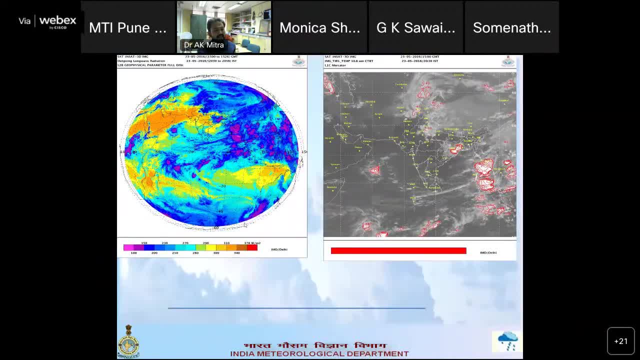 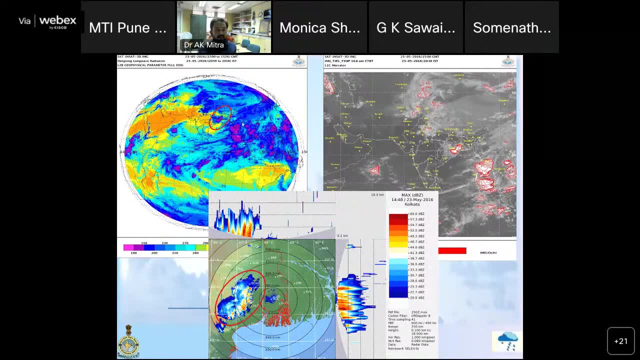 this is the calcutta reason. so, so, and then also, you can match up magic like you can. exactly from satellite imagery, you can find out. you can see the circle which i am drawing up, exactly the same phase of olr and ctt. you may get it and then, and then you'll finding out. the advantage is that. 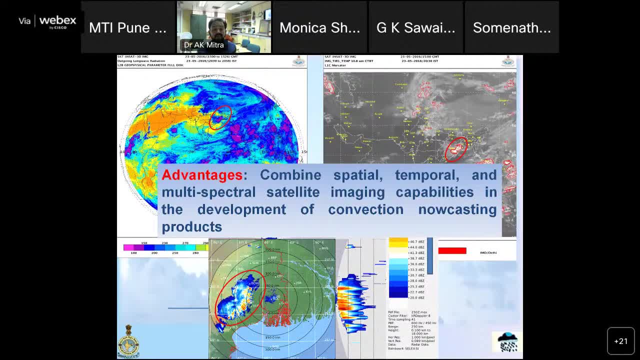 combining this spatial, temporal and multi-spectral satellite imaging capabilities, that is the most useful for development of convection, now casting products, so that here space tool or satellite plays a very important role. now some of the tool, like thunderstorm, if you can click on, like brick. 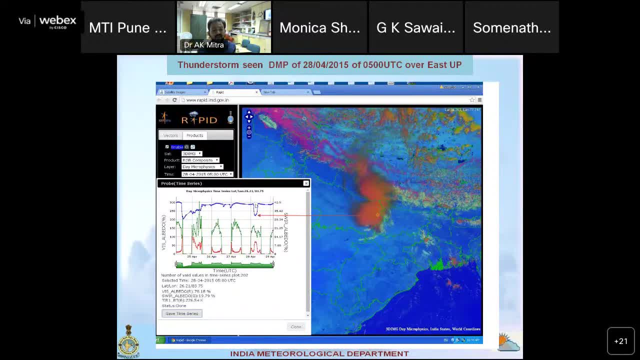 color or the eastern, eastern, utah, for this you'll be able to see that. you can see that you can see, you'll be finding out. there is a sharp grid, sharp uh declination of your temperature. there you can be advised. it can be issues that they're supposed to be from the thunderstorm and then some of the 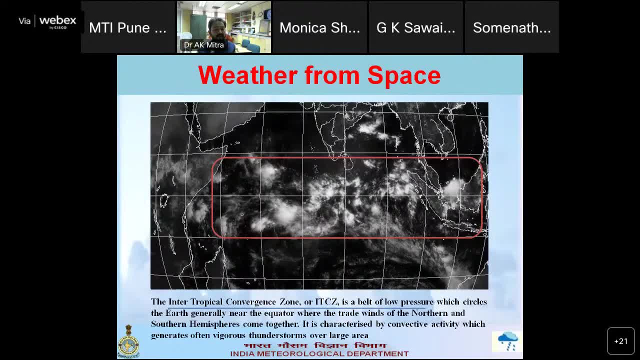 um some of the weather information that is, from the weather space you can find out intra-tropical convergence zone, that is the belt of low pressure which circle the earth, generally near the equator, where the trade winds of the northern and southern hemisphere comes together. that's the most important part, because this, this entire circulation, these itc get plays. 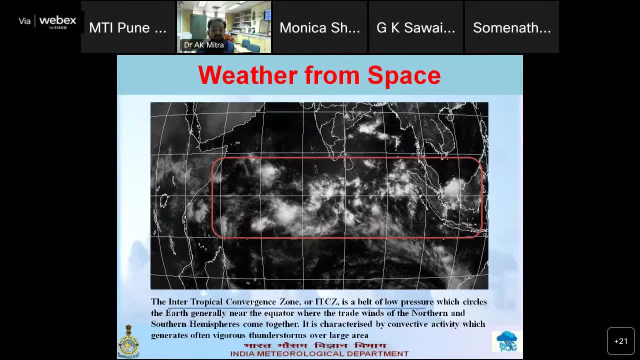 a very important role because it characterized by the convective activity which generates often thunderstorm over the larger area. for india mainly this itc that plays a crucial role for the monsoon and thunderstorm reason, and then this is the itc here from the ir and then western disturbance. 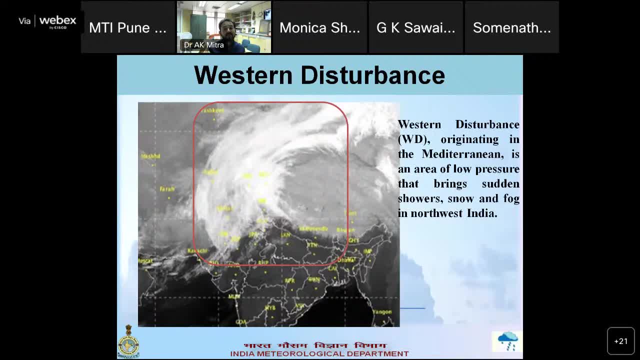 particularly during the during the winter. north india western disturbance, originating in the mediterranean, is area of low pressure that brings sudden showers, snow and fall for northwest india. so shape will be like this: you might have here when that is the western disturbance, and then, if you can see the thunderstorm here you 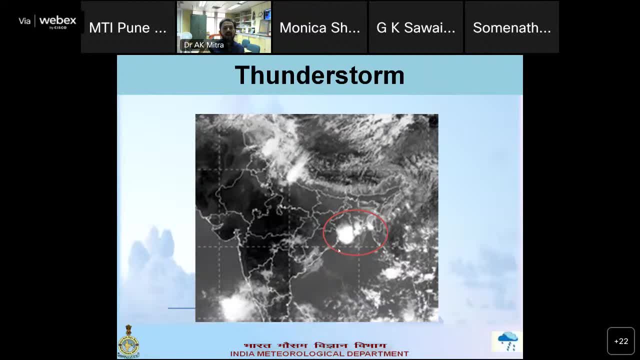 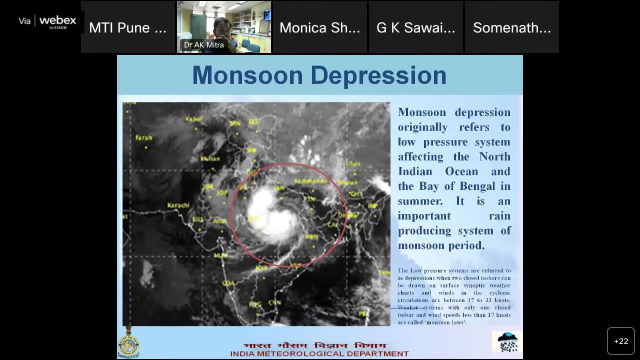 can see here this small, small thunderstorm cloud. this is the, the higher reflectivity values where thunderstorm can be seen. this one, and then it comes to the monsoon. depression during the during the monsoon originally refers to the low pressure system affecting the north indian ocean and the 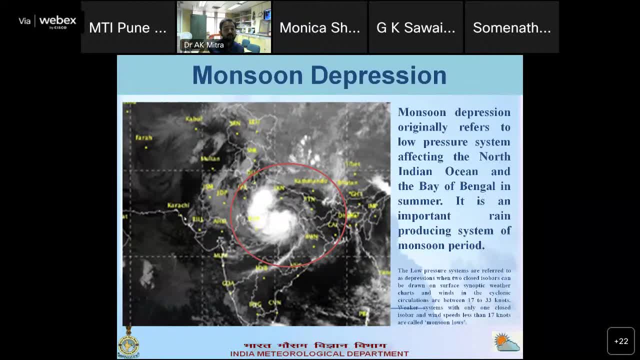 bay of bengal. in summer it is an important rain producing system, monsoon period. as you know, that low pressure area conform in the arabian sea or bay of bengal. we assume that it could be a. it could be giving a very lots of rain because it is a low pressure system and and this depression is 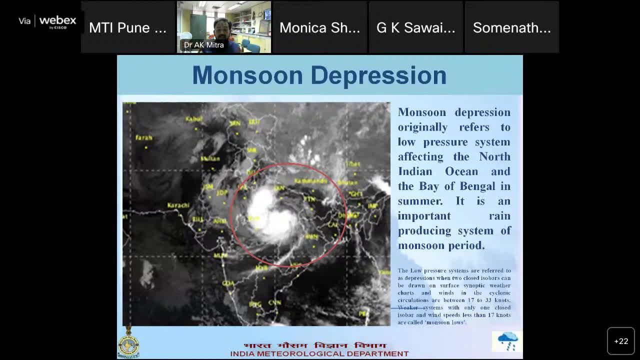 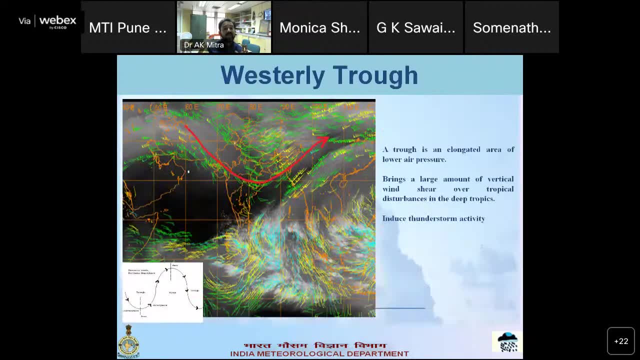 actually isobar drawn in the surface synoptic weather chart and the cyclonic circulation this will be will be around 17 to 33 knots. so this is the monsoon depression and then this is a westerly trough. that is also from satellite. you can get it because stuff is nothing but. 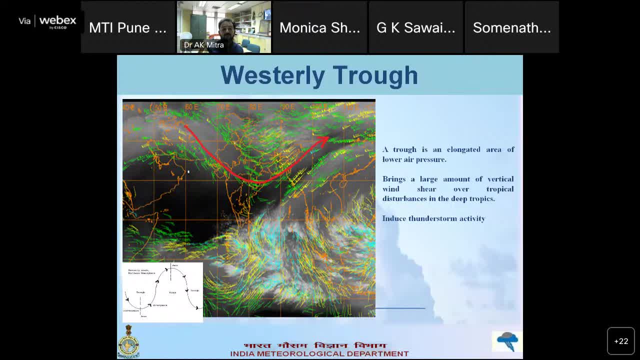 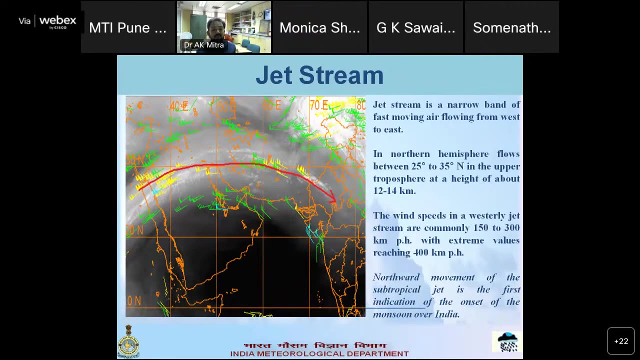 elongated area of the air pressure, lower air pressure. so they bring amount of vertical wind, shear and tropical disturbance and deep tropics and basically they induce the thunderstorm activities. and then this is the jet stream. jet team is the fast moving, you can say the best to east and north. i mean northern hemisphere between 25 to 35 degree north. 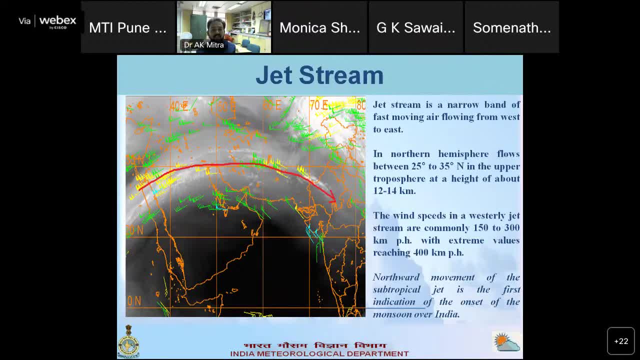 and height of about 12 to 14 kilometer, and this wind speed is westerly. jet steam are commonly 150 to 300 kilometer. so northward movement of the subtropical jet is the first indication of onset of monsoon over india. so the northward, so during the, during the monsoon period, it moving to the 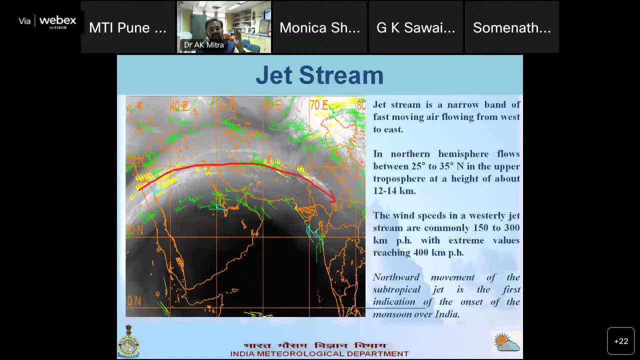 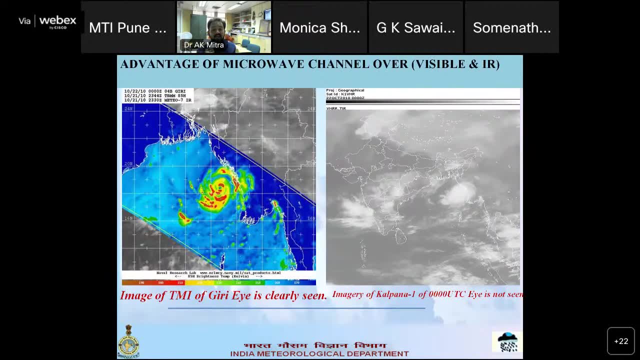 northward and during winter period it will be jet, steam will be lower. the southern, southern, southern world movement will be there. and then this is the advantage of microwave. see right side. you are seeing the um one expert time. just would like to again here now, whatever thing. 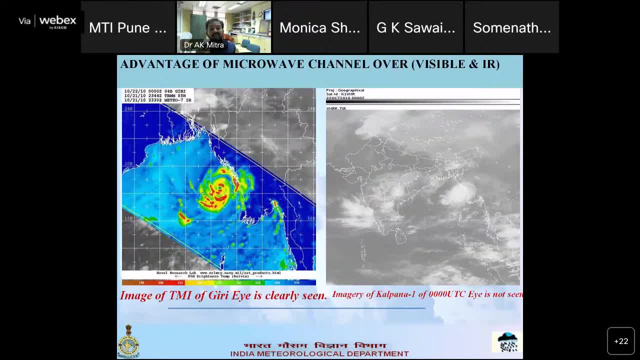 that is the imagery part that is from geostationary but sometimes, as i mentioned that, from microwave. what role they can play? now you can see there is one satellite of giri where ir imagery. you can't find anything from this right side, only only the the texture pattern. but here you can. 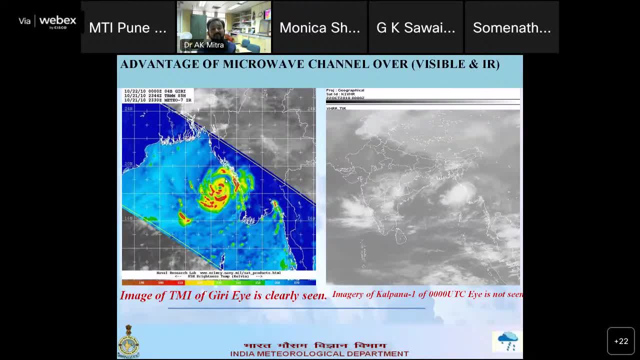 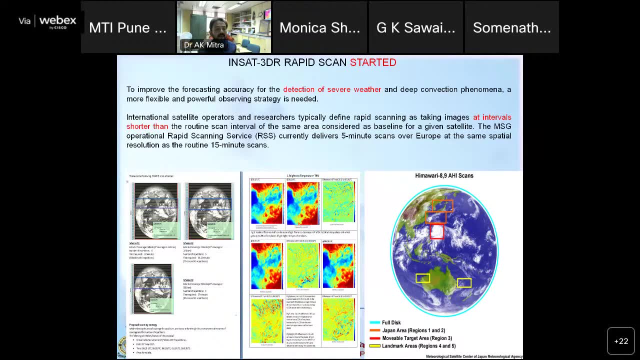 get. the entire initial internal structure of the cloud can be seen from the polar orbiting satellite. even if you can get one or two passes, it will help you. and then instead 3d. 3d are rapid scan. basically, as i mentioned, that every scanning is the most important because it gives you the 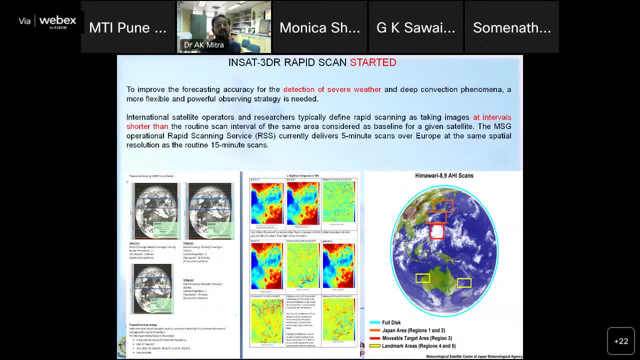 temporal resolution to improve the forecasting accuracy. detection of severe weather is most important. deep connectivity is more important and powerful observing tool is scanning the earth at very higher interval. imd has started from segment division for and half minutes rapid scan and that is roughly around five minutes for indian reason and you can see here this is a country sop we have. 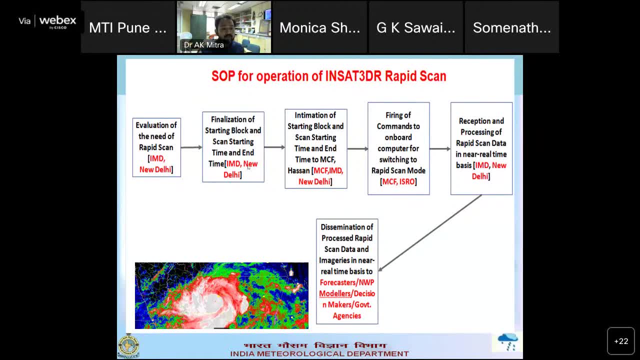 made from the forecaster as we got to know the area we tried to build up this in, and then it will go to the mc of hassan and then we disseminating this particular portion of the observation to the forecaster, nwp modelers, decision maker, government agencies, and then you can see. 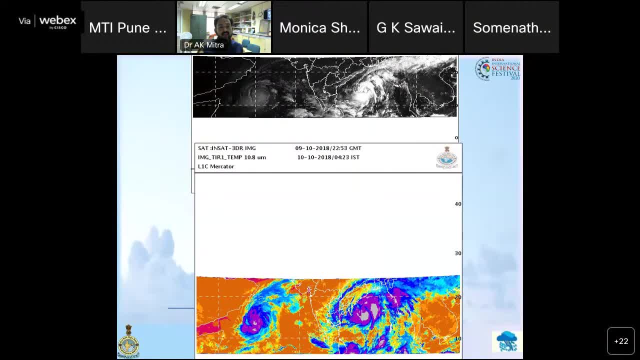 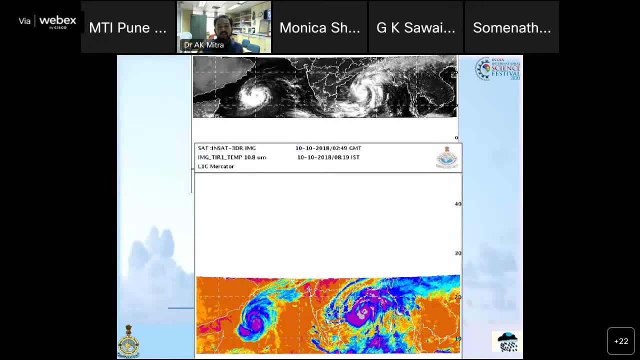 here. this is the animation of this rapid scan. you can find out here that how rapid scan plays. they're not two cyclone were there at the time that year 2018. you can find out every four and a half minutes. you can see the both the satellite at every four and a half minutes, very high. 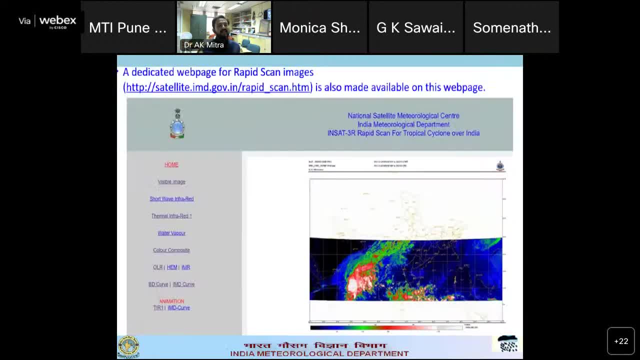 temporal resolution. we have a dedicated web page for this rapid scan. you can get into- uh, you will get it all: visible image, shortwave image, thermal, infrared, water vapor, color, composite, olr- all the information of the rapid scan you can get it. let me tell you this is the most important. 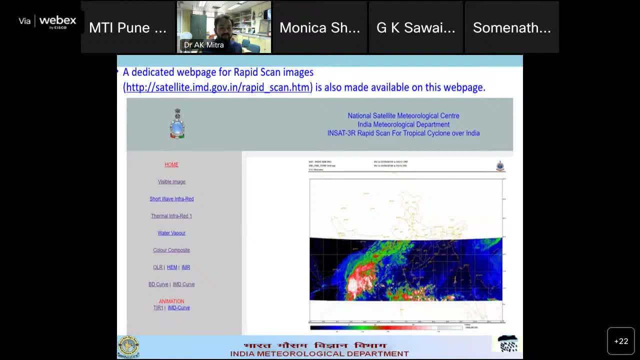 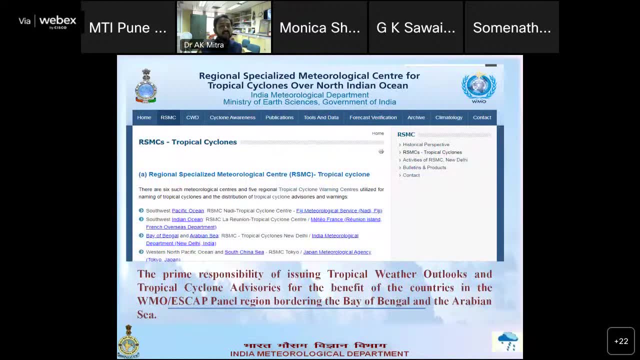 very high temporal resolution, rapid scan strategy and then, like you can see, the vsc and lubon and titli, as i was showing you the animation, so you are getting it. and then original specialized metallurgical center. uh, as, madam, as a previous speaker has already mentioned that this is a 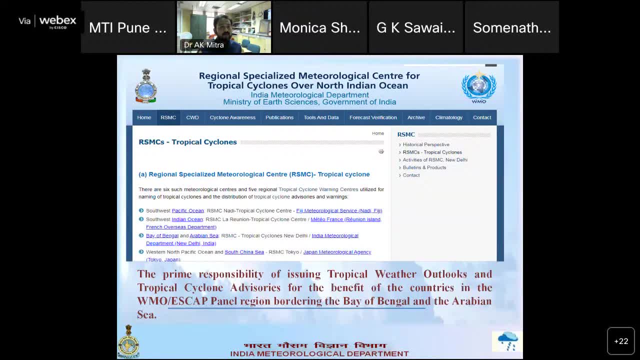 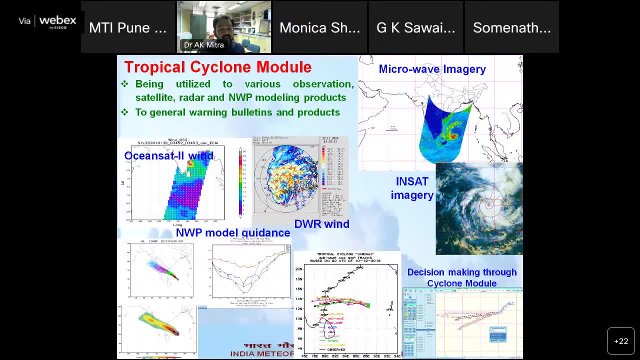 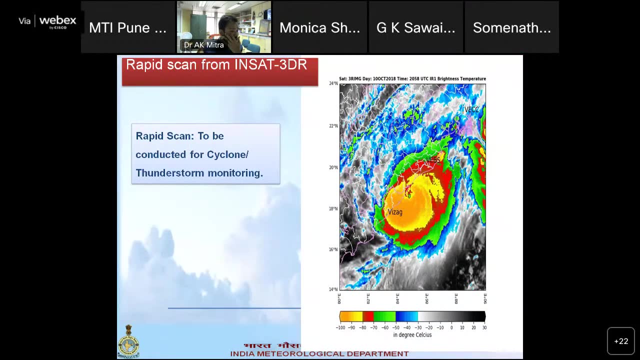 there we are, we are, we are getting this information designated to them and these are the tropical cyclone modules, like number of microwave inset. so all our satellite drive product, where the decision making is the most important, crucial role from space is is one of the inputs, like you can see here, uh, instead 3dr rapid scan um. i can also be seen in. 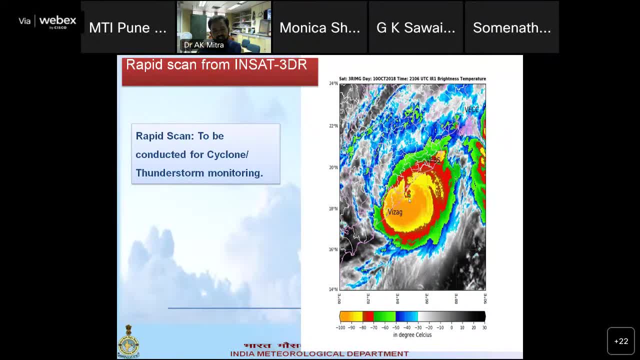 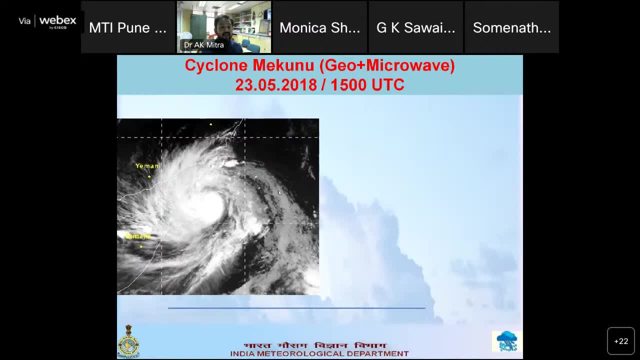 the green color, you can see the animation. like you can see, this is one. so this is, this is the kind of a tool which will really help us a lot. and then this meccano: you can see uh one cyclone and this one. so, left hand side, you can see the imagery where uh ir imagery during night time, but either 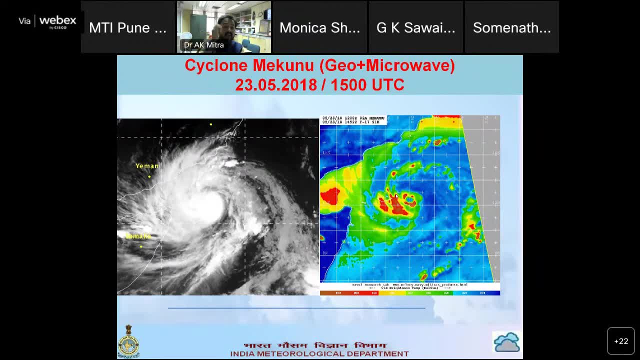 right hand side you can see. the microwave imagery will give you the internal structure. now what basically internal structure means. internal structure will give you the the information about whether the cloud liquid water content is available near the wall cloud or not, because intensity will be defined by the wall cloud also here. so there, you can see here, but where is the? 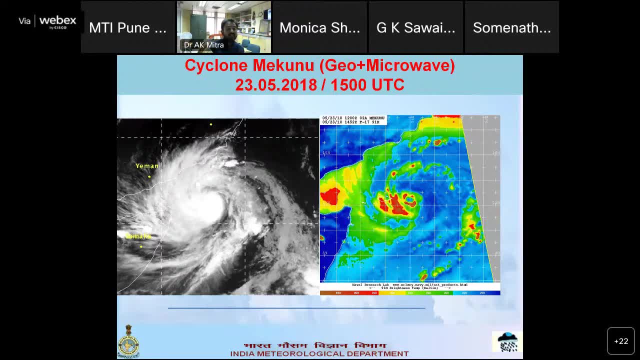 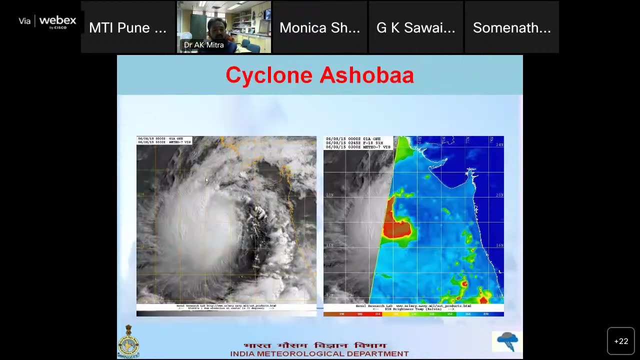 geostationary. you can't make out this thing because in ir there is a, there is a. there is a shortcoming that you cannot get. you are getting only the cloud top temperature, but in a microwave it can penetrate through the clouds and that can give you the information. and then now this is a similarly asoba cyclone. you will be seeing that. 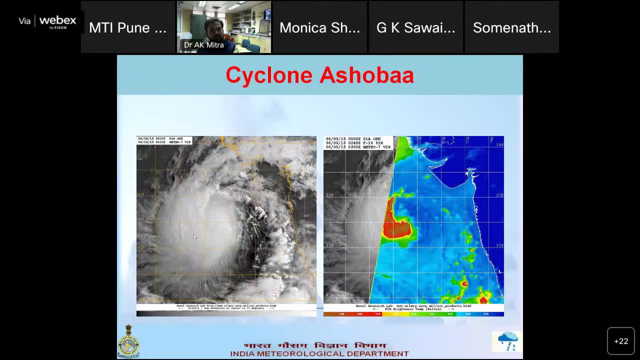 left hand side there is a complete intense cloud patch, whereas in the microwave we can see the internal structure of heavy drain band or you can see the kind of water liquid content option over scatter metric wind. you can see the the higher the signature of the black one that we can. 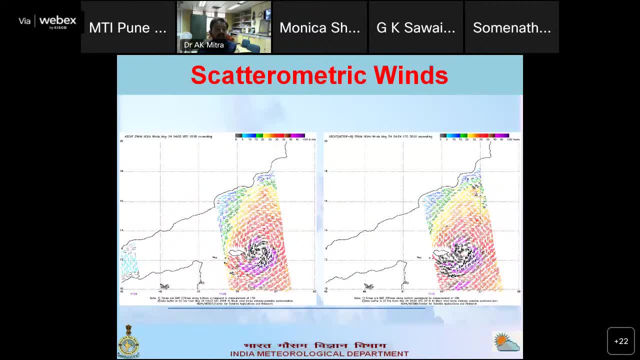 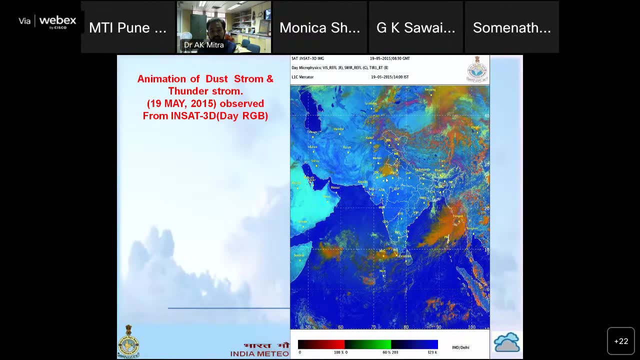 see. intensity is very high. the scatter metric wind is also very important- from the escape- and this is the animation of dust storm. you can see here the dust storm. you can see here. now you can see the cloud. this dust is moving from jodhpur. you can see from jessalmer jodhpur. 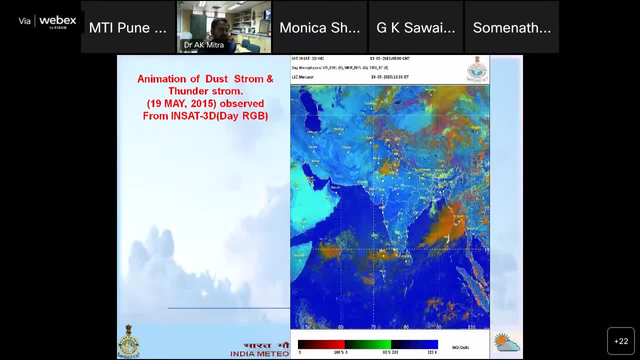 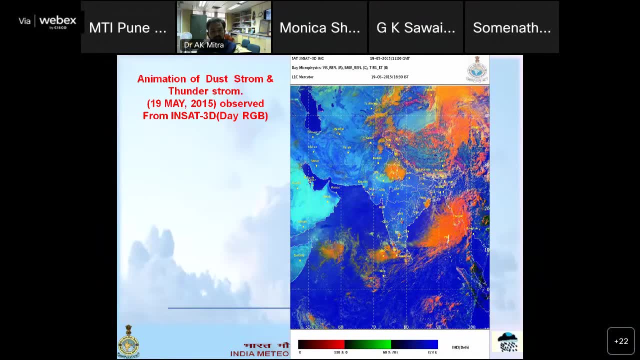 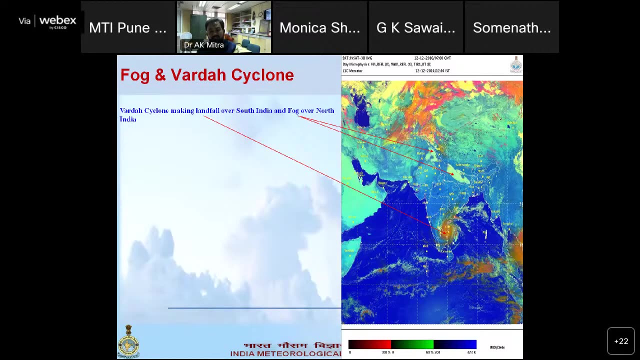 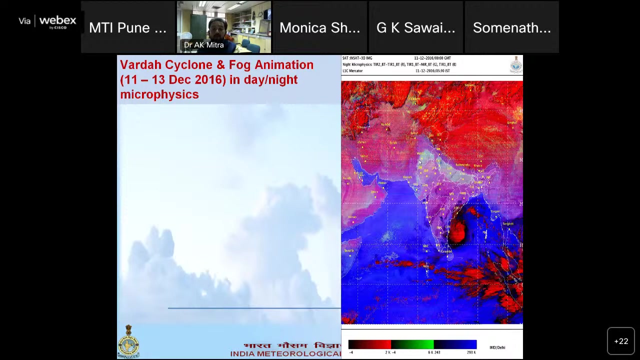 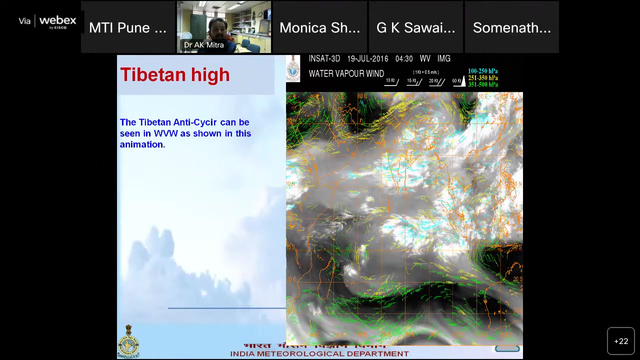 it has all started. so here the rgb is the really greatest tool we can say the last five, six year we have been get benefited our observation, as there is a. there is a real improvement from this and this is the kind of the high you can see, where the tibetan plateau, where anti-cyclonic circulation can be seen from the 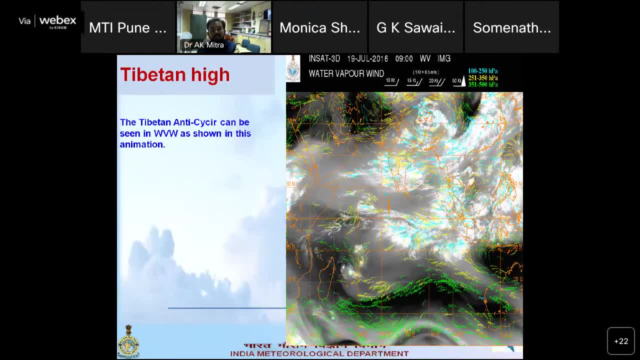 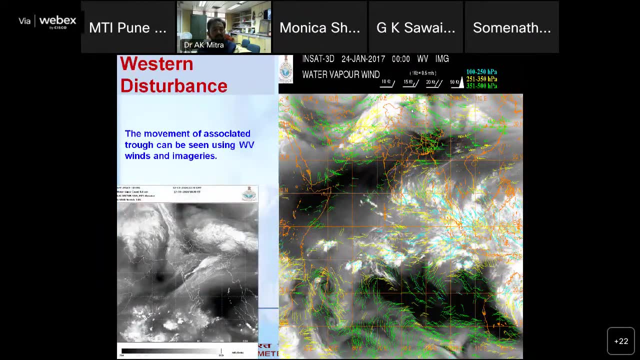 water vapor channel and with the animation so that, anyway, this is, this is the kind of information which is most, very important for the forecaster wd that you can see approaching wd with the help of approaching wd 560 ahead. it can be given northern india that can. 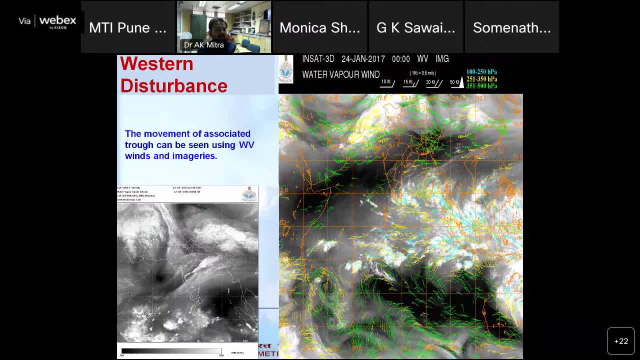 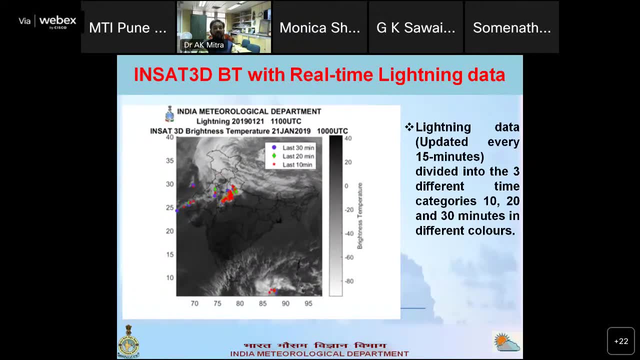 kind of advisory that parts of a area would be affected by rainfall, thunderstorm and lightning, and this is the one example of how lightning has been merged. from md website you can see the lightning data has been updated with the satellite imagery and all you can say: merge with and it is. 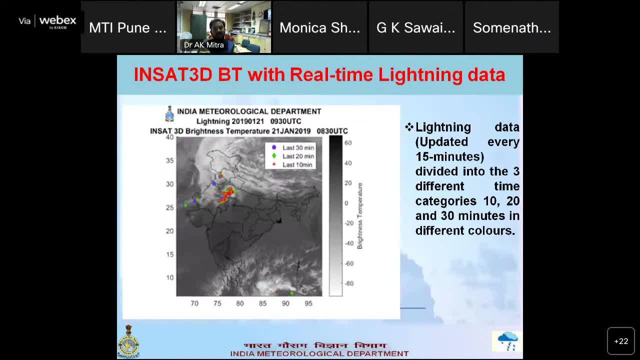 the most important for indian air force, iitm and all these things we gather together from isr and imd. we made it here in segment division. we formulated in almost three, four, i four, three, four years and it is a very good, crucial knowledge about the 10, 20, 30 minutes of the 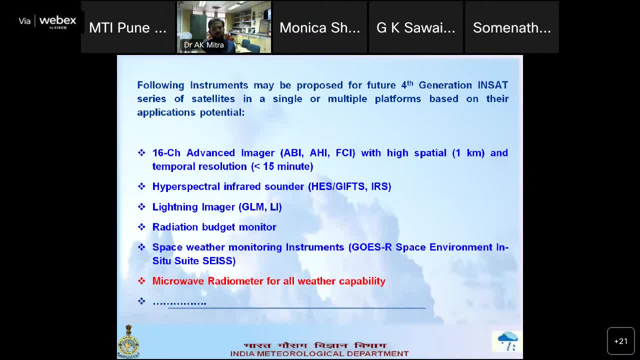 different lightning occurrence from. instead, 3d- and this is the proposed fourth generation satellite- is 2025, where at once the major- as i'm mentioning that for human satellite- we can get it. then hyperspectral infrared sounder is also very useful. now we have a broadband sounder, but there 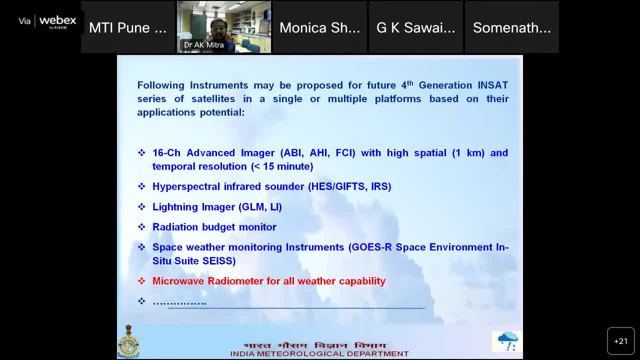 we need, our requirement, is hyperspectral sounder, then lightning images over the satellite, like what goes is having radiation budget monitoring, space weather monitoring instrument and microwave radio meter for all weather capabilities. so these are the proposed features for generation series of satellite uh. with the multiple platform we are approaching from isro, let's hope, and this is i'm thankful to. 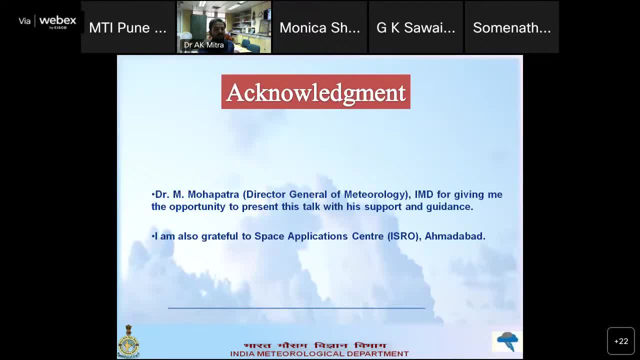 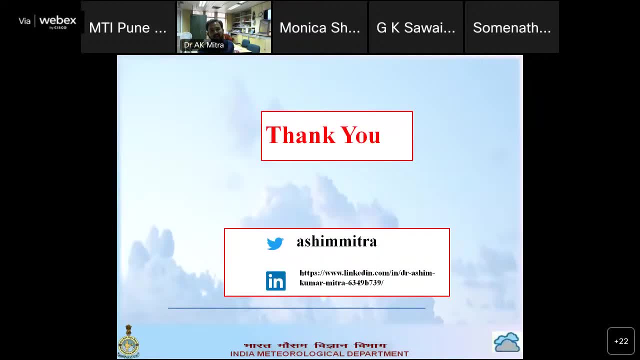 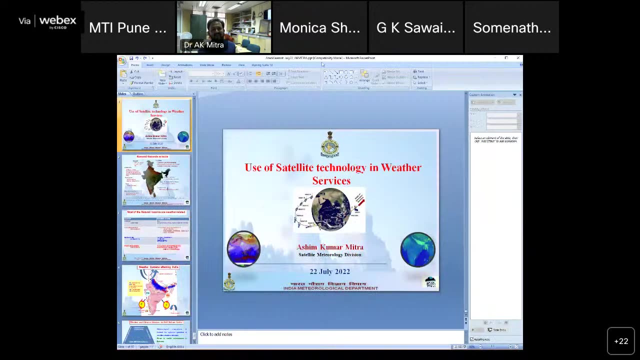 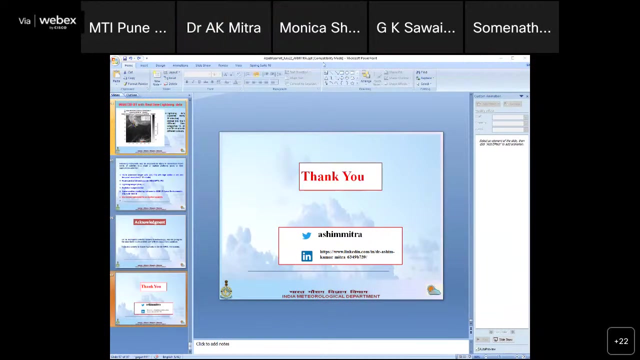 all, dr mafadrasa, our tgm sir, for giving me the opportunity to present this talk. thankful from israel and all other my colleague and and other sources where i can, i presented this one. thank you, uh. i thank dr mitra for his very informative and excellent lecture. uh to the audience, if they have. 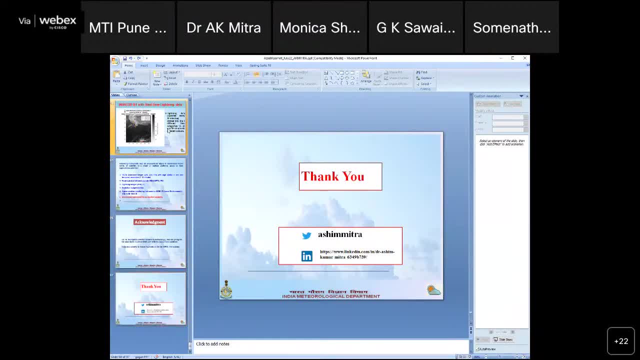 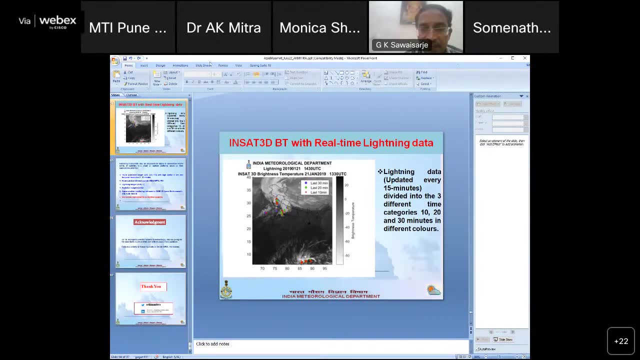 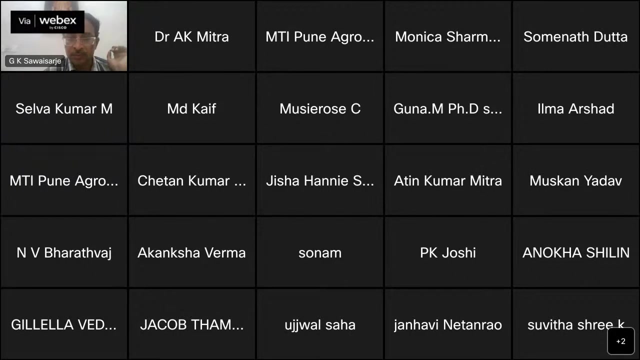 any queries they may, please ask. they may also write in the chat box. still, we have five minutes, so we will continue with the next lecture, thank you. so i request all the audience to freely ask questions to dr mitra. some of the participants like atansha chetan kumar. 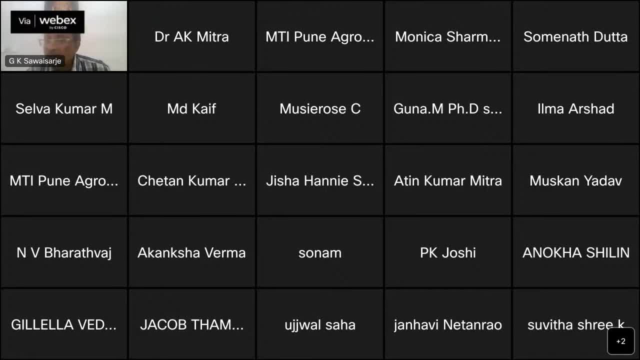 uh, yes, uh. one question from the chat box to dr akimitra: how is wind data obtained from remote sensing? so there is a question. yes, i think this is a very good question because, uh, there are a different way of getting this wind data from satellite. first, is the from geostationary satellite wind data has 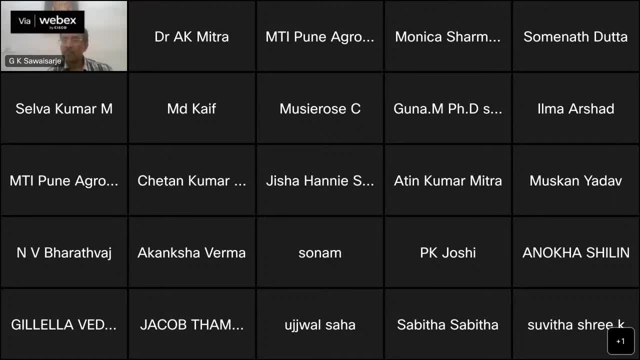 been derived from geostationary consecutively three images. so there are three images like: if i want to derive from eight utc data, then seven thirty eight utc and eight thirty utc. these three imagery has been aligned. after aligning it, we are getting the um, the pixel which is being uh, which is being moved. 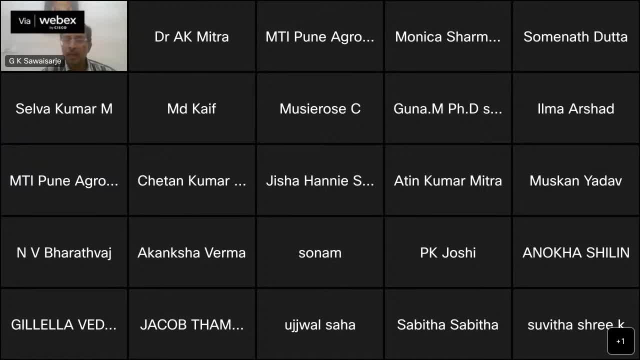 out, moved out. you can say the cross correlation method has been employed, so there is a huge system. but i would say the cross correlation method of movement of the cloud can be can be calculated with the velocity of the velocity of the movement of the cloud, like 20 meter per second or 20 km per 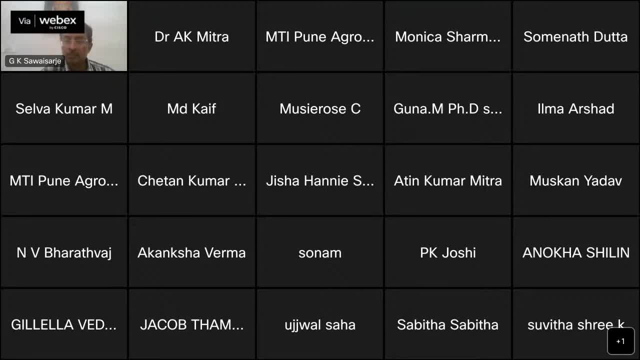 second, the way we are calculating and then algorithm assigned which height will be assigned to that cloud from that nwp model. first case was taken and then derived from the geostationary satellite, whereas in a polar orbiting satellite it has been captured from different way. it is: 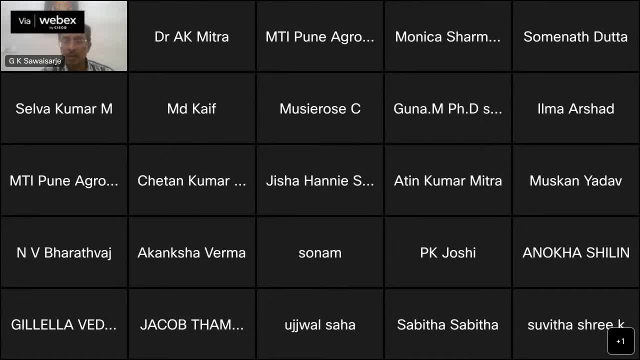 there is a direct method of beam where the microwave um you can say horizontal and vertical, you can say the movement captured from the microwave satellites. so geostationary satellite consecutive images are required from the polar satellite are directly connected to impact boundaries. From the polar satellite there is a single calculation of the computation of the wind. 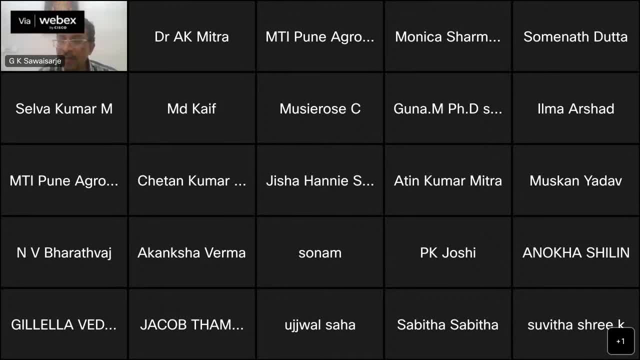 Okay, There is another question from Tushar Pawar. Why don't we have ozone column measurements over India with the help of remote sensing? Ozone column measurement we have basically from INSEAD 3D, 9.7 micrometer is basically. 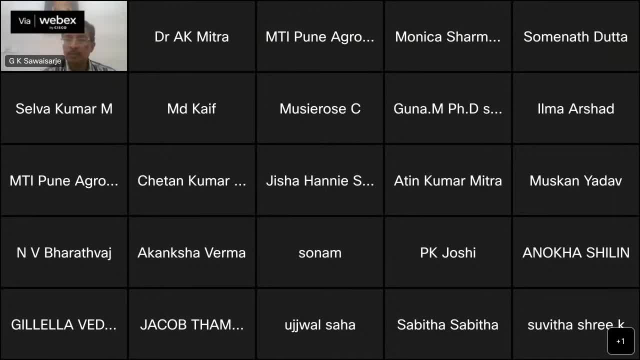 detect the ozone channel. yes, we are getting it. ozone column, we are getting it here. The important part is that from geostationary perspective, the accuracy is not, as that may lie, on the- compared to the microwave. So in the microwave, yes, microwave ozone column is much better than the geostationary. 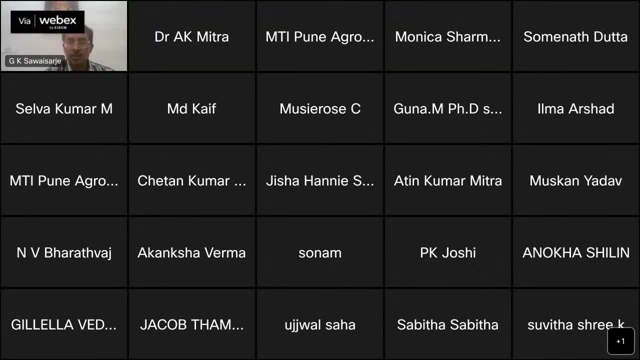 because a lot of you are. you can see the mid-level of corrections of your different constituents of gases and then the transmittance. So these are the things are like you know, but from geostationary also you can calculate it. 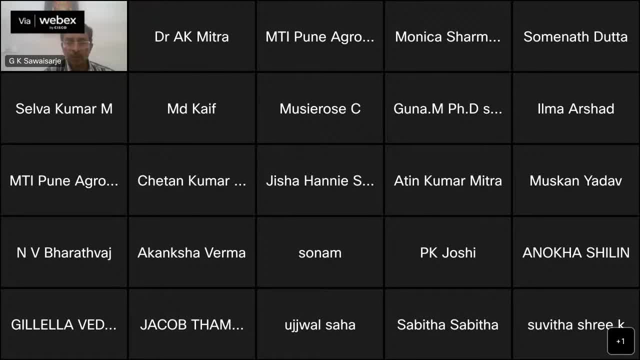 But microwave it is the most Okay. Any questions, still questions from audience? they may please ask. Okay, I think there is no more questions. I thank Dr Mithal for his excellent, informative lecture And the audience may feel anytime they may contact Dr AK. 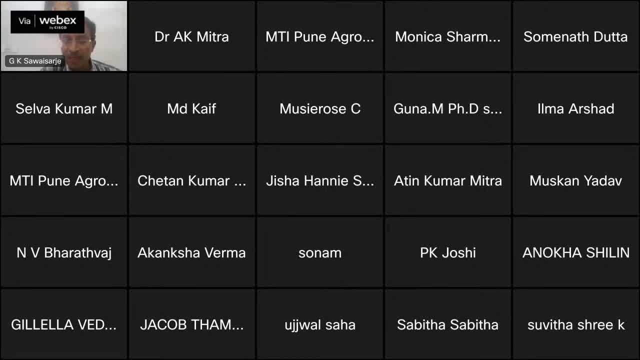 Mitra, he is in SACMED division at our headquarters, Delhi, So for any queries you may please refer him. Okay, Thank you, Thank you. Thank you. Okay For the audience. next lecture will be on next Friday, coming Friday. 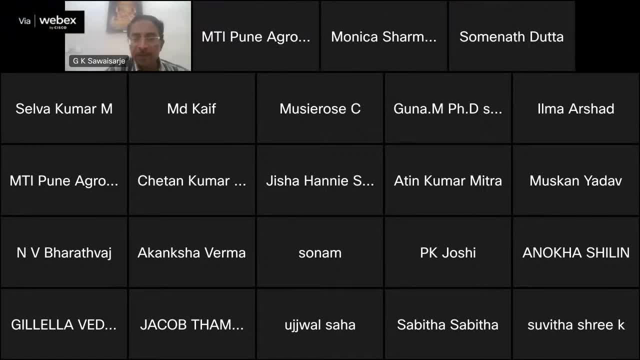